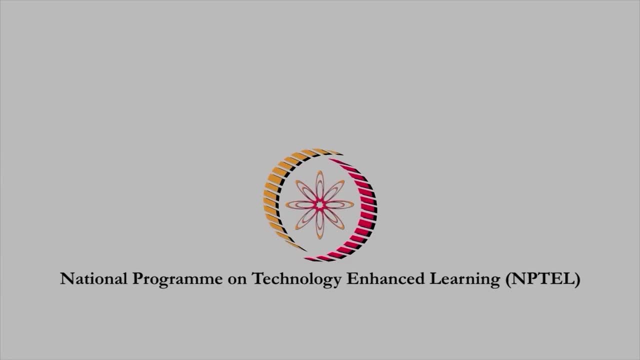 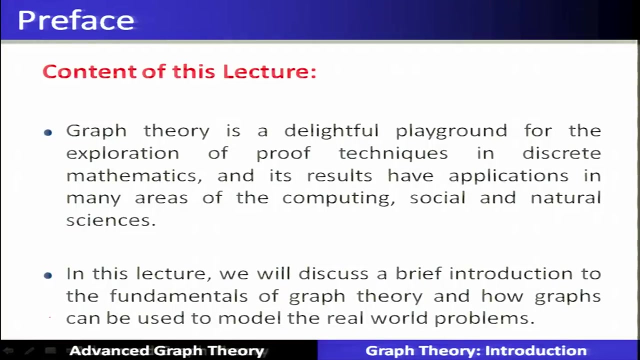 Graph theory. introduction, So content of this lecture. So graph theory is a delightful playground for exploration of proof techniques in discrete mathematics, and its results have applications in many areas of computer science, social and natural sciences. In this lecture we will discuss the introduction and fundamentals of graph theory and how the graphs can be. 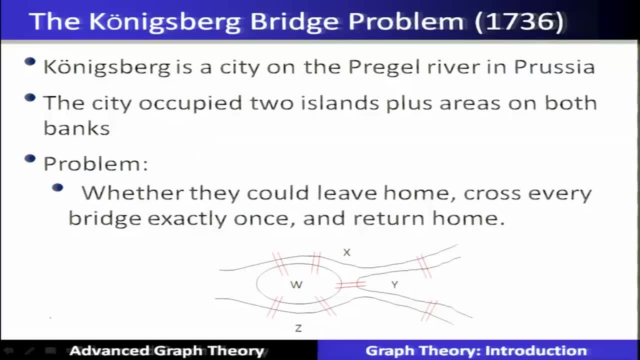 used to model the real world problems. So the graph theory is evolved out of a practical problem of a Konigsberg bridge problem in 1736.. Konigsberg is a city on Prigel river in Prusia. The city occupied two islands plus areas on both banks. So the problem. 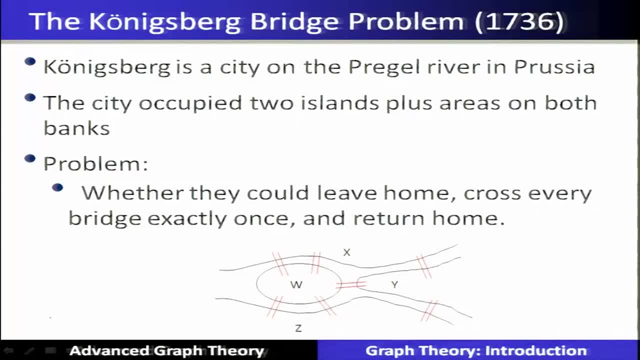 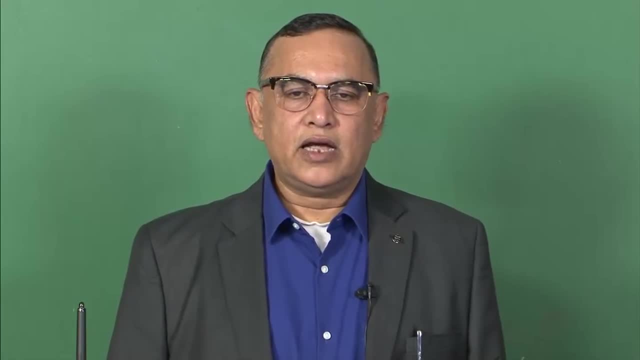 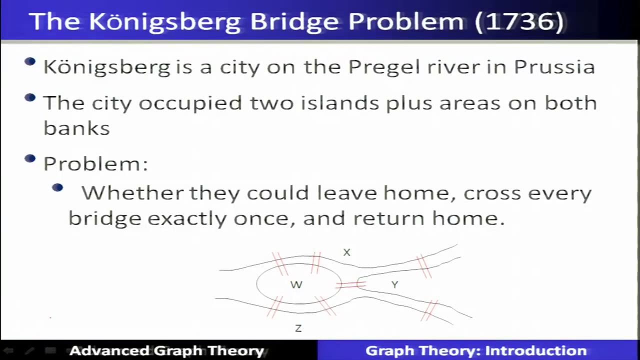 was stated as under whether the residents of that particular city they could leave home, cross every bridge exactly once and return home back. So in this particular figure can see that x, y, z, w, they are basically the islands and these islands are connected by. 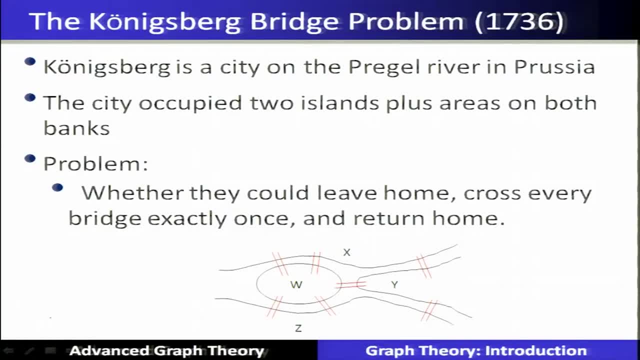 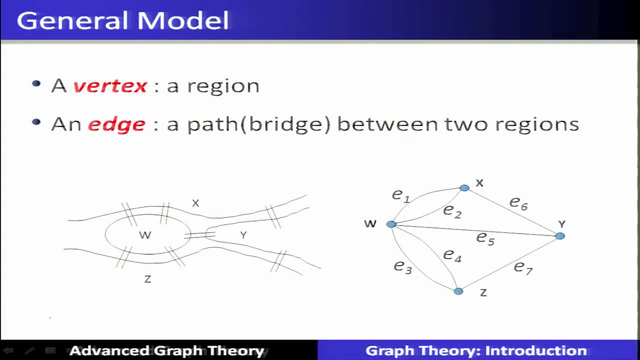 the bridges which are marked by the double lines which are shown in red colour. Now, this particular problem can easily be analyzed if they can be modeled as a form of a graph. So that means every region or a island if we can represent as one of them. So you can see that k 2, k 2 plus h 2 plus h 4 below it. 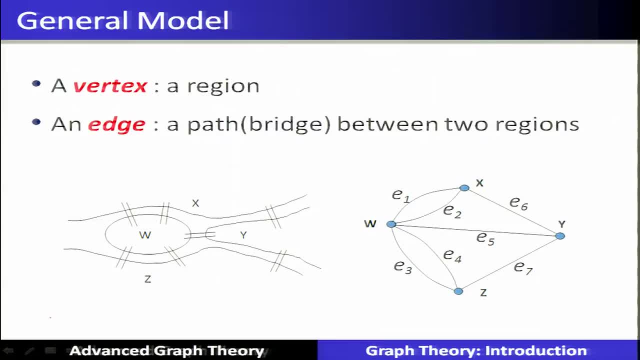 a vortex, and then if there is a bridge between the two regions, connection or connectivity, then basically we can place an arc. So this particular map is basically converted in a form of a graph. So here you can see in a particular graph. Now, once a problem is converted in a graph form, then this particular problem can be analyzed. 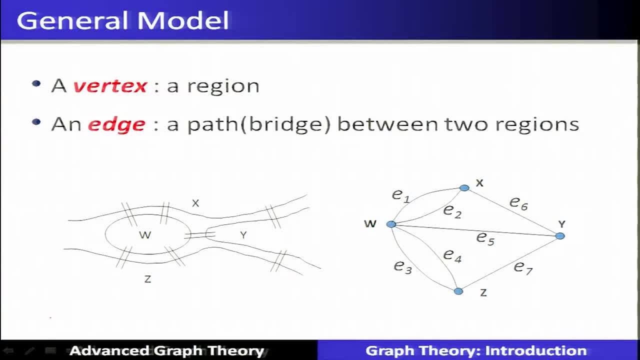 using the model in a graph theory. So this is the way the most of the practical problems or the applications, if they converted into a form of a graph, then basically the problem can be analyzed and solved. in this particular lecture We are going to see how different applications can be modeled in this form of a graph and 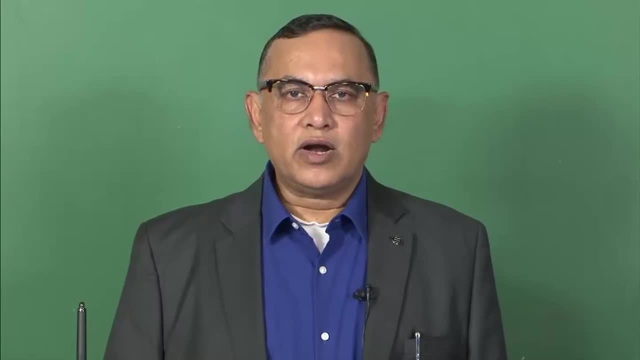 that is called a graph model. Once a problem is modeled in a form of a graph, then basically we are going to study in this part of the course the theory that is a graph theory and which is based on the proofs, and various techniques and the algorithms are based on these particular methods. 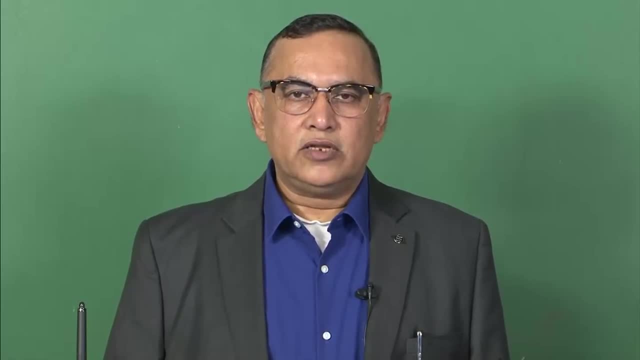 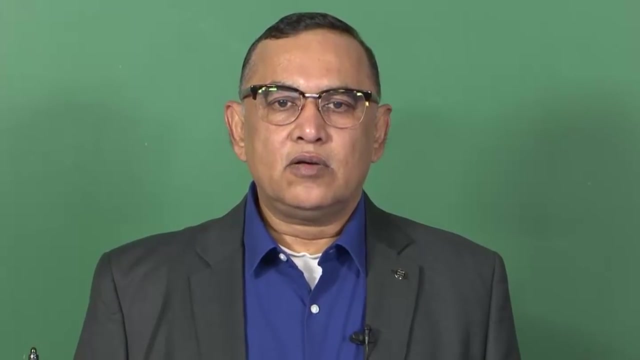 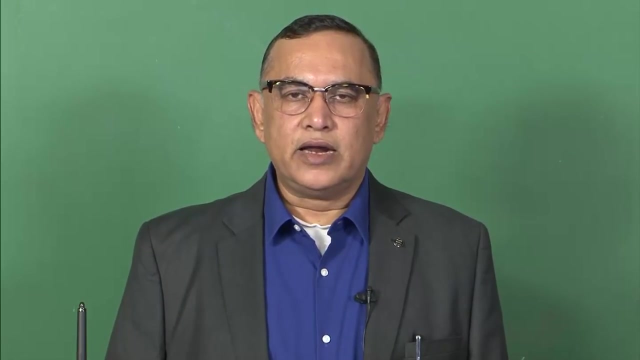 So, as far as the algorithms are concerned, which are basically covered in this, graph theory is going to exploit the structural property of a graphs and how they are going to be represented in a computer, that we are going to see How the graph can be represented in a computer form, in a memory, so that the algorithm can 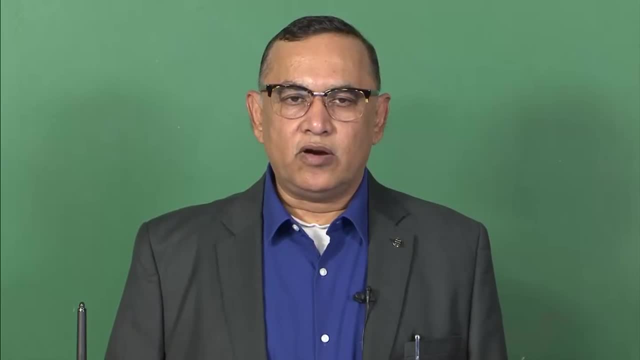 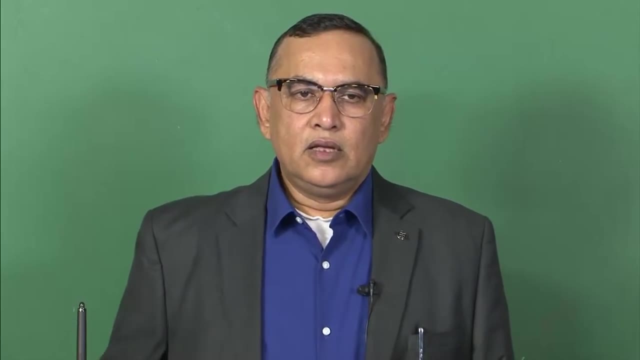 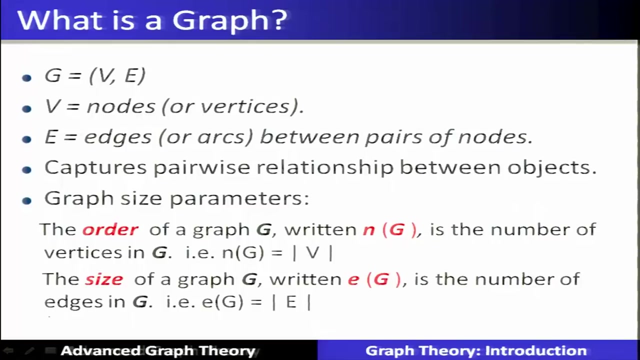 exploit this particular model that is called a graph model. So let us see in more detail about the graph. So what is a graph? So graph is a pair of set of vertices and a set of edges. So graph G is represented as V comma E, where V is a set of nodes. 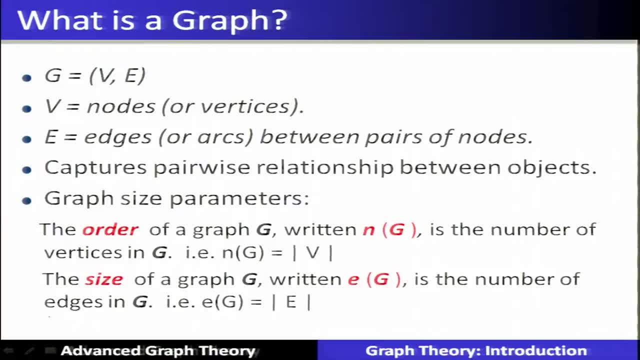 And E is a set of edges. So set of edges is nothing but the pair of nodes. So this particular graph will capture the relationship between the vertices, also called as a objects, and these arcs represents the relations between the objects. So different applications will pose these relationships and we are going to get a graph. 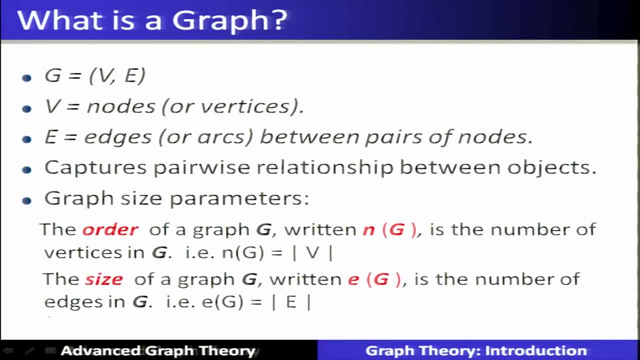 as a model of different applications. So this particular graph, once it is defined as V, comma, E and represented as a big G, then this particular graph has different parameters and we basically call a graph with those parameters like the order of a graph. G we can represent as the total number of vertices present in 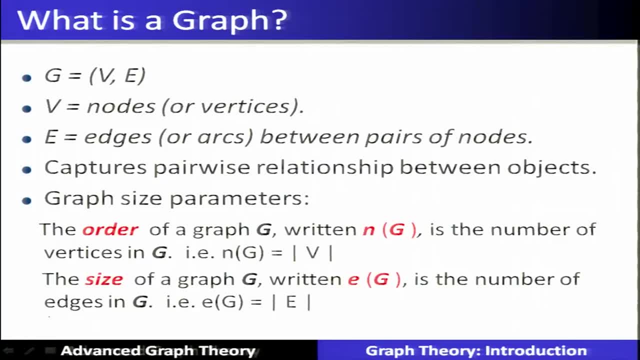 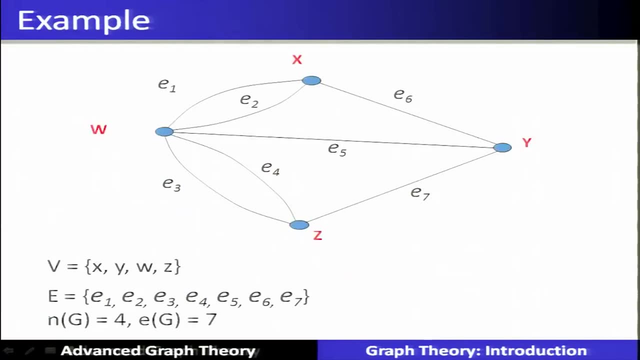 the graph. So when? Similarly, Similarly, the size of a graph, which is represented as the number of edges in a graph, is basically the cardinality of the edges, and order of a graph is the cardinality of the vertices. So they are basically the graph parameters. 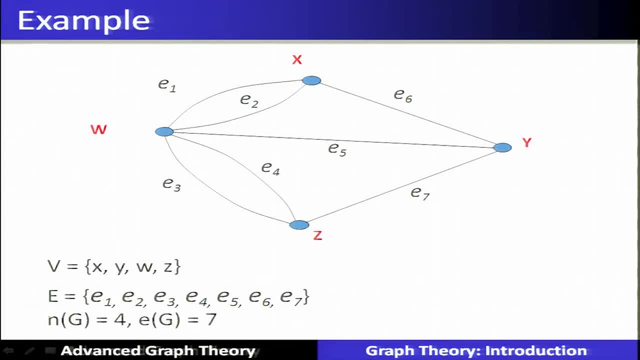 So in this particular example of a Konigsberg bridge problem, which is converted in a form of a graph, we can see the set of vertices. they are number 4 different vertices. the order of the graph is 4.. Similarly, the size of a graph is 7, because there are 7 different connections or 7 different. 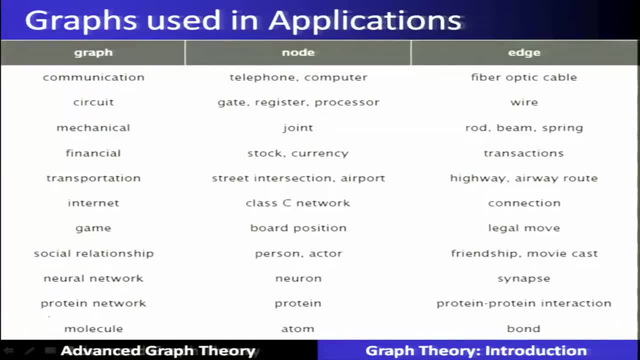 bridges which are connecting those vertices, Like we have seen, a Konigsberg bridge problem- that particular problem was modeled as a graph. So graphs we can now see is being modeled for different other applications. So the applications and how the graphs are being formed we are going to now discuss briefly. 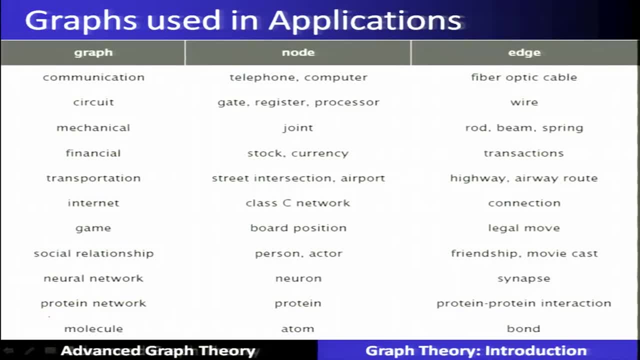 all of this. So, as far as if it is a communication network, then the graph which we form out of a communication network, where the nodes represents basically the telephones or basically the other instruments, equipments and edges are nothing but the cables which connects these particular end. 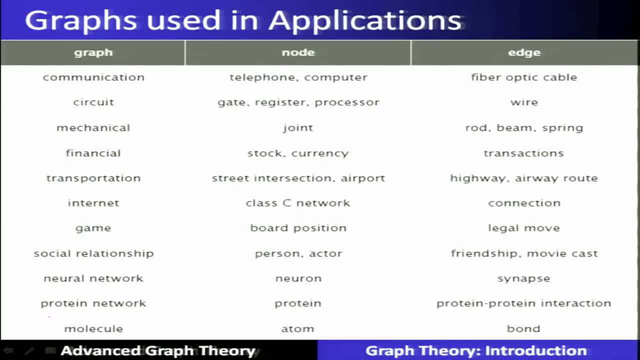 equipments. So that is called basically the communication graph. Similarly, let us see, Let us see, Let us say, the transportation graph comprises of the nodes. nodes are nothing but the intersection points of a road, or basically the airports, and the edges are nothing but the arcs which 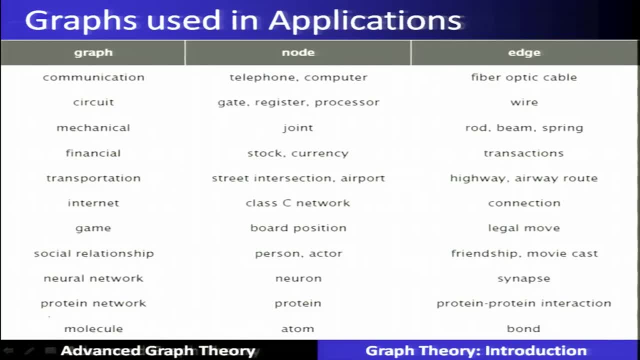 connects these intersections or basically different airports connected by the flight. So this is called basically the transportation network. whether it is a road transportation network, you can represent as a graph. Similarly, the airline or air connectivity of a particular nation you can represent, also in a form of a graph. 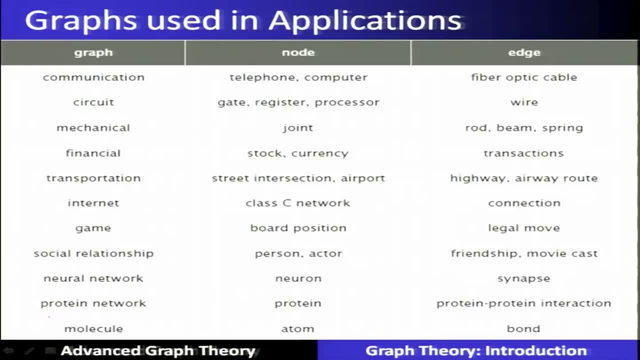 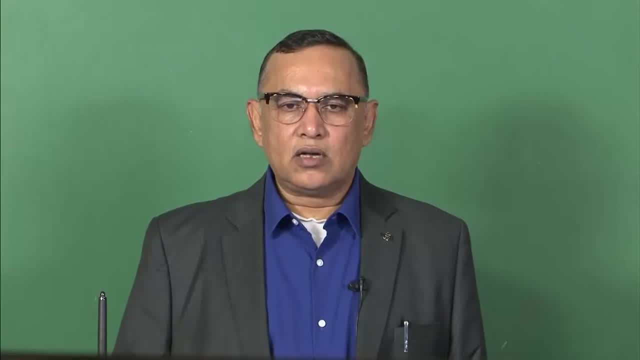 Internet also, you can represent in a form of a graph, where the node represents the classy network and the edges becomes the arcs or the connections between these classy networks, and this all will evolve into a internet and that can be analyzed Similarly. the social network. 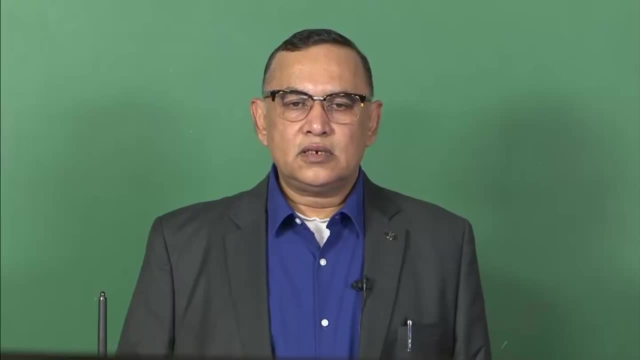 Where, Where, Where, Where Where Is because the north then knowns the actors or a persons, and the arcs represents the friendships or the relationship or acquaintances. So such networks are basically, which are used in a social network that is called for. 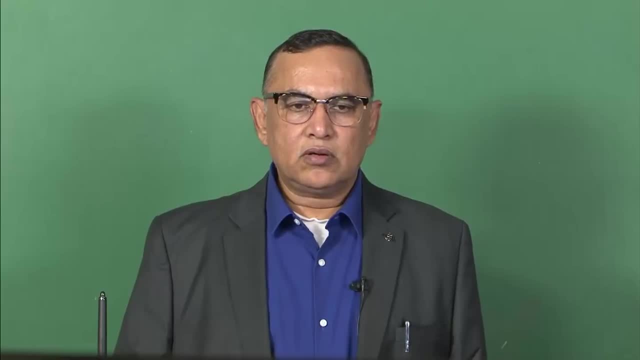 social graph. Similarly, neural networks also can be basically modeled in a form of the graph where the nodes are nothing but the neurons And the arcs are synapse, So that every has two. like Mic, Swedish social network, Protein networks also. similarly we can be defined: 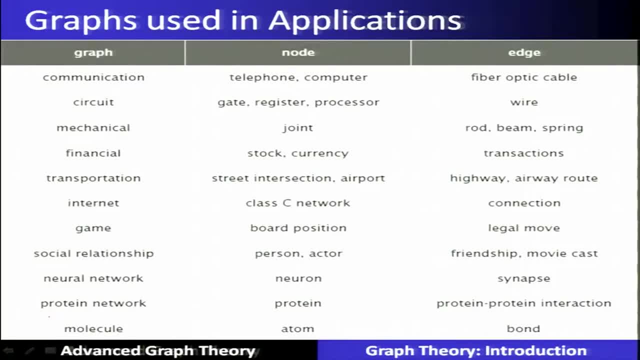 So you see that there are applications- almost most of the applications- where the problem you can model in a form of a graph and do the analysis and solve the problem. So once a problem is modeled in a form of a graph then you can visualize the problem. 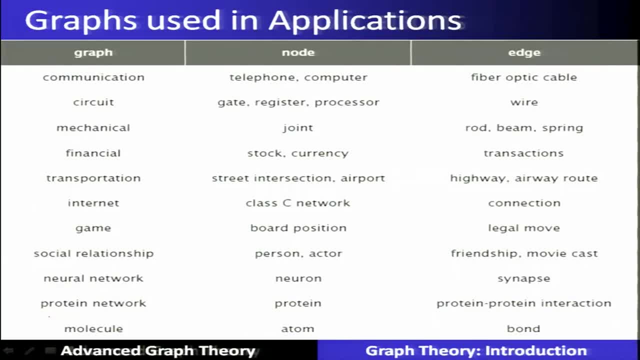 and applying the theory of a graph theory, which we are going to cover in this part of the course, can be used to analyze the problem and solve problem more accurately. why? because lot of theorems and the proofs are available, So those can be used to solve the problem correctly. not only that, we can also develop. 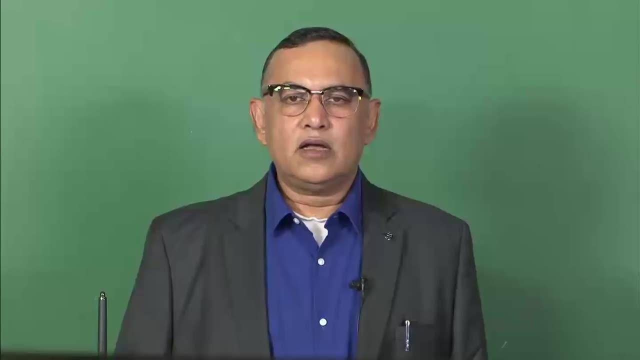 the algorithms, once the graph is represented in a computer, how it is represented in a computer that we are going to see, Once the graph is represented in a form of a computer, and the theory. using this, that particular theory, we can exploit the structural properties of a graph. 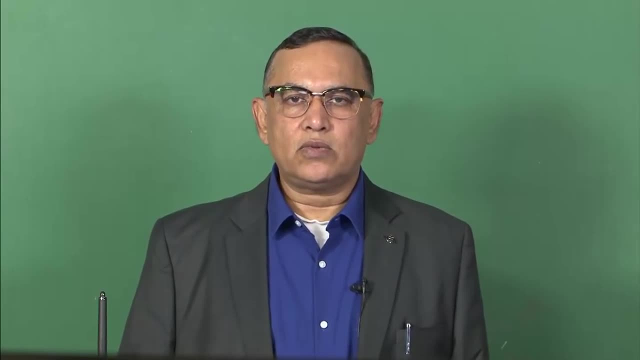 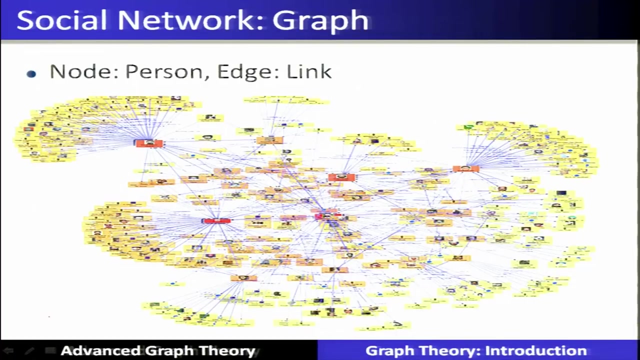 So in this part of the course, the algorithms which we are going to discuss will exploit the graph structural properties to solve the problems which are there in the applications. Let us see the example of a social network. So what is the graph here in the social network? 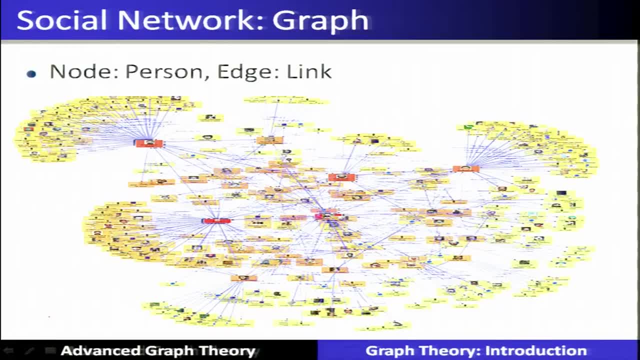 So the nodes represents the persons or the people, and the edges will represents the link between the people or relations between the people. So the social network graph will look like as per shown in the figure. it is a big graph which will form, which will keep on evolving where the nodes will come and new nodes are. 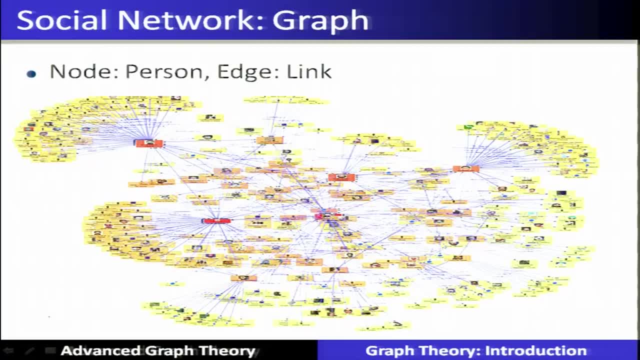 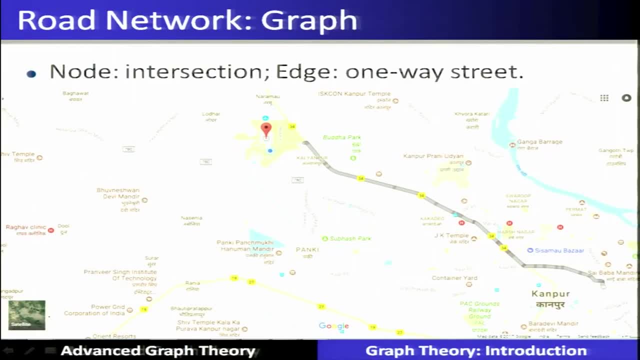 joining the network. So network, social network keeps on growing in this particular manner: Road network. how it can be modeled as a graph we can see over here where the nodes are nothing but the intersections and the arcs or the edges are nothing but the nodes. 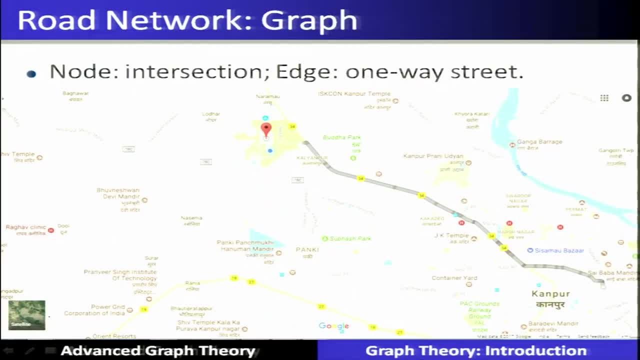 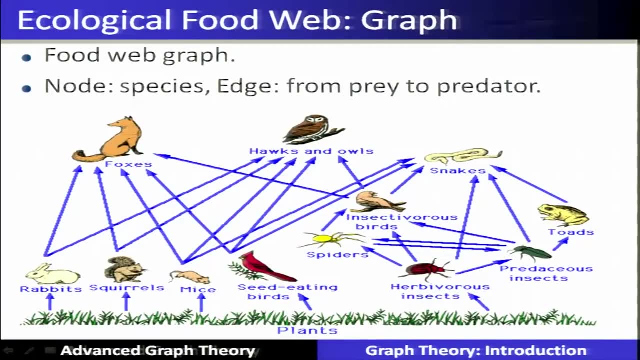 The road segment which connects these intersections. so we can form or we can evolve a road network and this can be modeled as a form of a graph. Ecological food web also, you can represent in a form of a graph, as a model, So wherein the node will represent different species and the arcs and the edges are nothing. 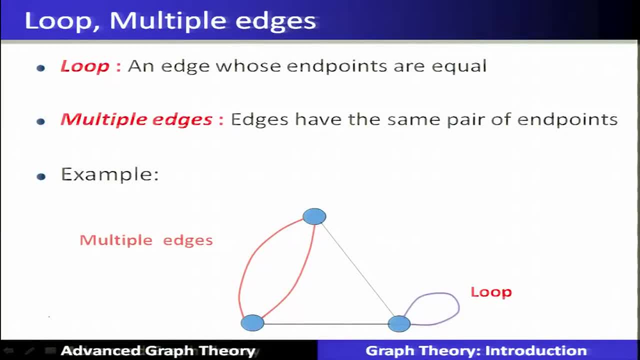 but the prey to the predator. Now, coming back to our graph, so we can see that if the edges or the arcs, which will basically have the same end points, or the end points, are equal in the arc or the edges, then it is called a loop. 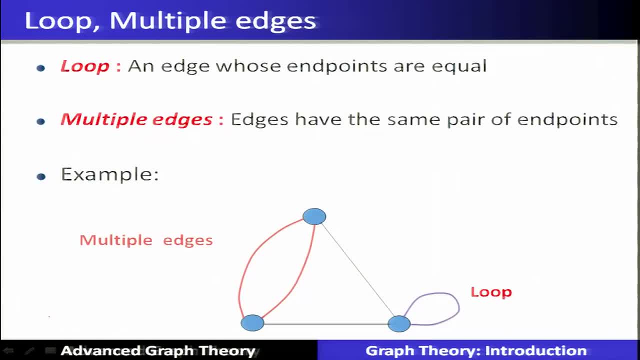 And if, let us say, the edges or the arcs have the same end points, more than one edges having same end points, called multiple edges. So it is shown in this particular figure. you can see here that this particular arc is basically the multiple edges And if, let us say, the edge is meeting at the same vertical, 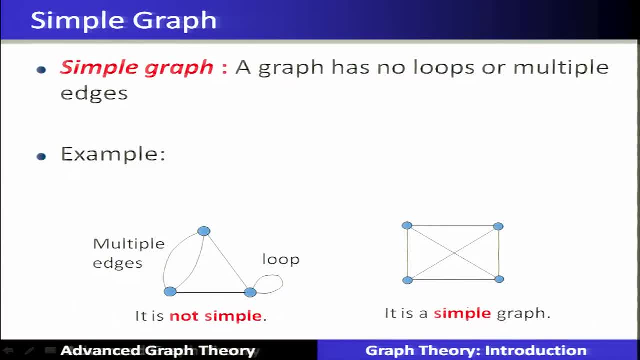 Vertex, then it is called a loop, Now a graph which has no loops and also which has no multiple edges. such graphs are called a simple graphs. Some people call them as a regular graphs also. So in this example on the right side, this is the simple graph. why? because it does not. 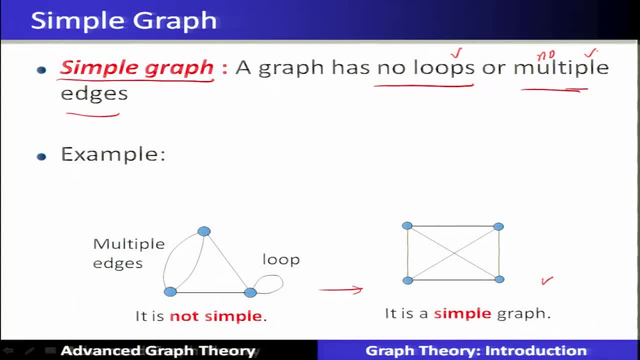 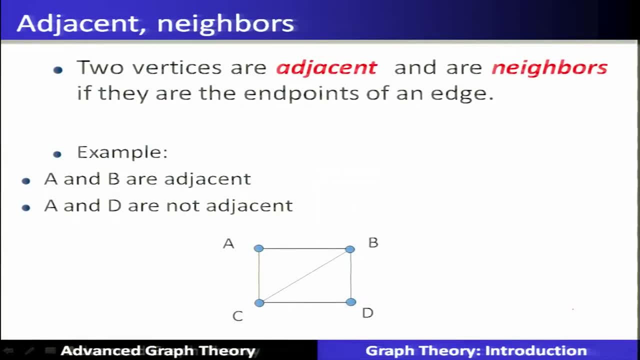 have any loop, nor it has any multiple edges. hence it is a simple graph example which is shown over here Now. furthermore, we are going to discuss if the edges are present in the graph. what does it means? So two vertices: if they are having an edge, then they are adjacent and also they are called. 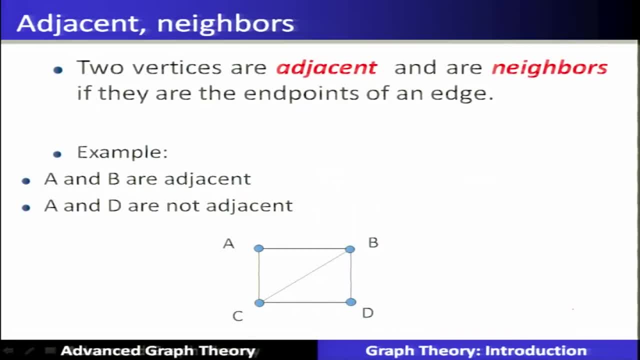 as a neighbors if they have the end points connected by an edge. So here in this example, A and B, they are called adjacent. So A and B are adjacent why? Because there is edge present over here Now A and D. there is no edge, hence they are not adjacent. 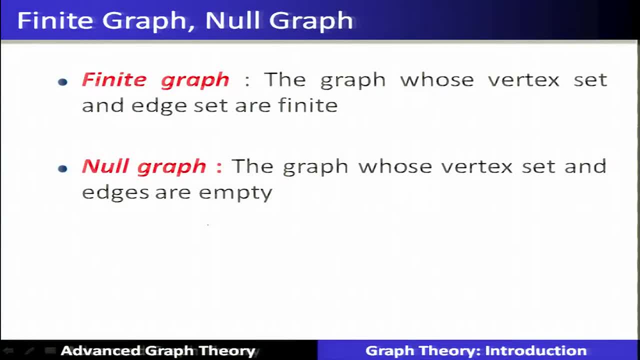 So finite graph, a graph whose vertex sets and edge sets are finite. that is what we are going to basically assume in this particular discussions. So null graph is the graphs whose vertex sets and the edge sets are empty. So null graphs are a trivial graph. we are not going to cover up those particular null. 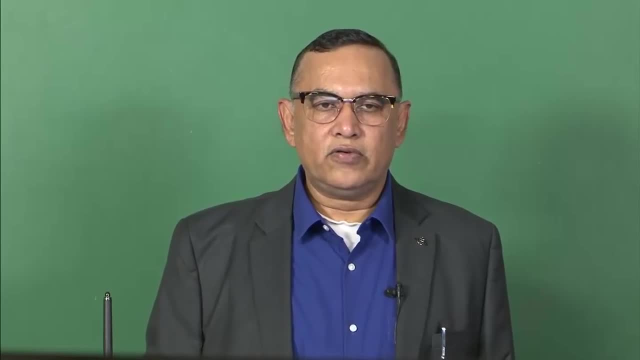 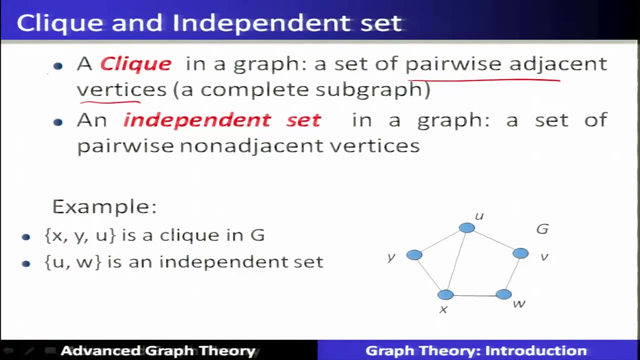 graph as a model in this theory of a graph theory. Furthermore, the set of pairwise adjacent vertices is called a clique. These are some of the terminologies which are going to be widely referred throughout this particular lecture. Now, a set of pairwise non-adjacent vertices is called independent set. 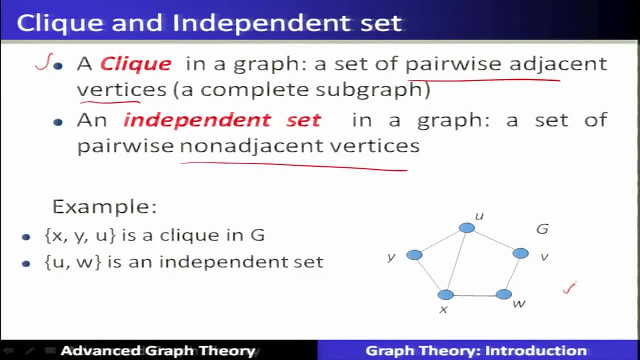 So in this example we can see that u, x and y, they are set of pairwise adjacent vertices. hence this is a clique. Let us say that these two vertices, v and y, they do not have any edge Hence. So this will form a set of pairwise non adjacent vertices and is called independent set. 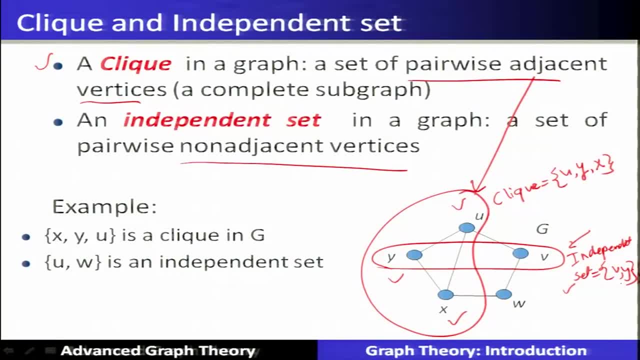 Now you can see, in this particular graph, you cannot find a clique which is bigger than this particular size, that is, more than the size 3.. Similarly, you cannot find an independent set in this particular graph example which is having the size more than this size, that is, more than 2, hence they are basically the 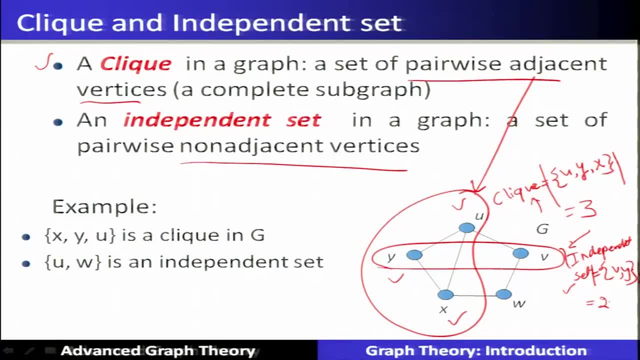 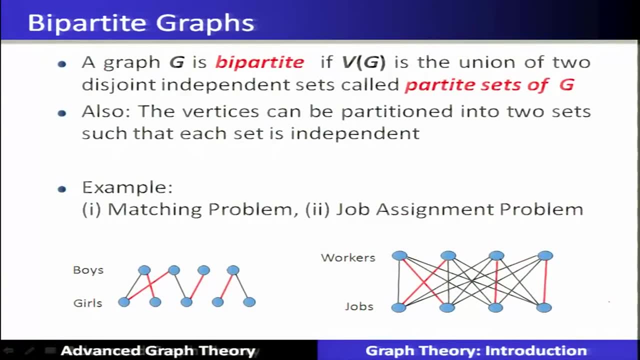 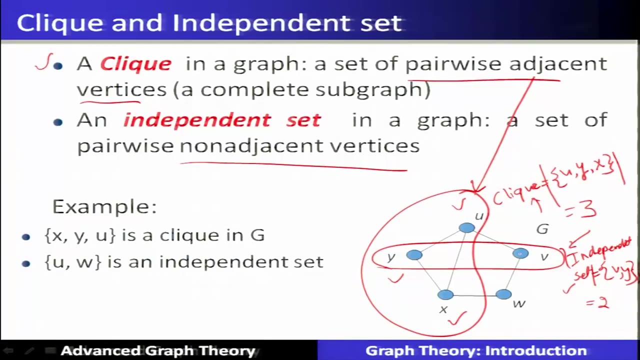 biggest or largest cliques. similarly, the independent set: it is a largest size independent set. Now a graph wherein the vertices are partitioned into two disjoint independent sets. Independent sets- I have already given you the example- which do not have a mutual edge. 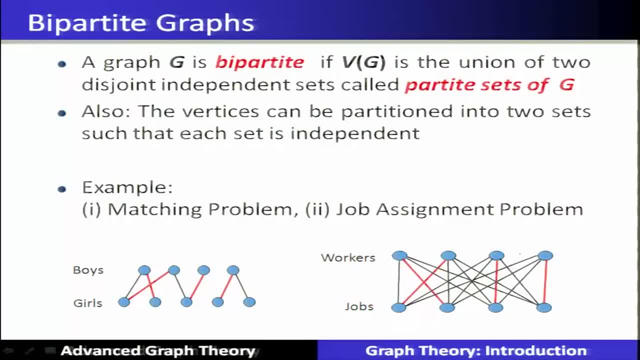 or they are pairwise non-adjacent vertices. so that means, if the vertex VG is partitioned as two disjoint independent sets in a particular graph, then that graph is called a bipartite graph. So partite sets of a graph means the independent sets of a graph. so if the graph has two partite, 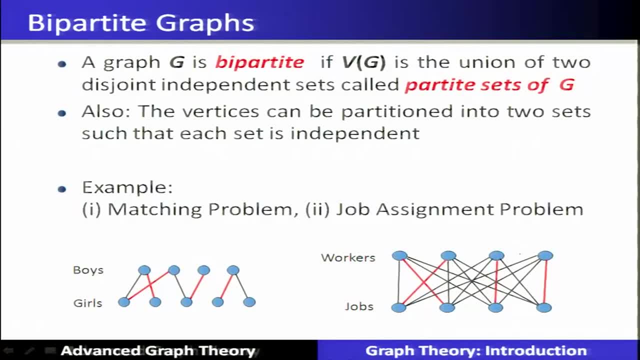 sets. So this is called a bipartite graph. Example we can see here: all the boys are represented in a form of a set and all the girls are represented in another partite sets, and the graph which we form is called a bipartite graph. 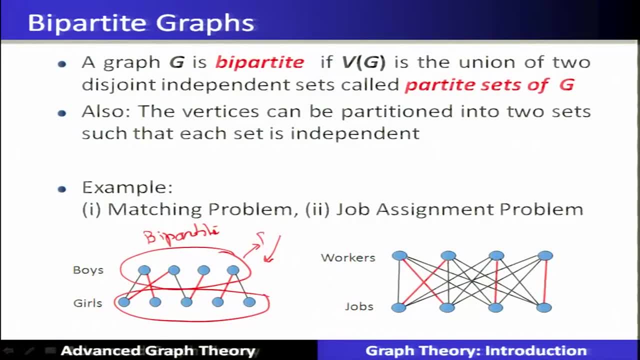 So this is partite set 1, this is another partite set. Similarly, if you are solving the job assignment problem, that is, the placement problem, so here, in this particular applications, we have the set of jobs which can be represented as one partite set and the set of workers which can do a particular job will form another. 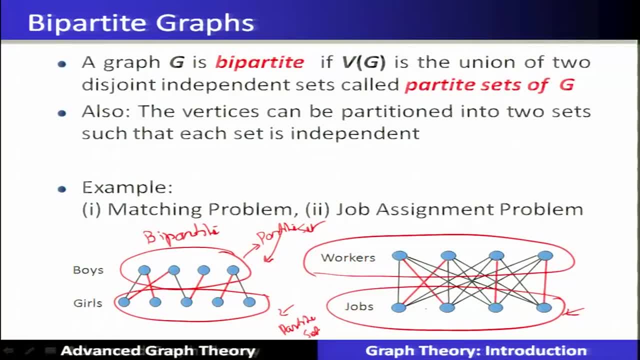 partite set. So the graph which will form out of their relationships is called basically the bipartite graph. So bipartite graph is going to be very useful wherever this kind of applications where two different partite sets are there and we require a graph to be analyzed with such a relations. 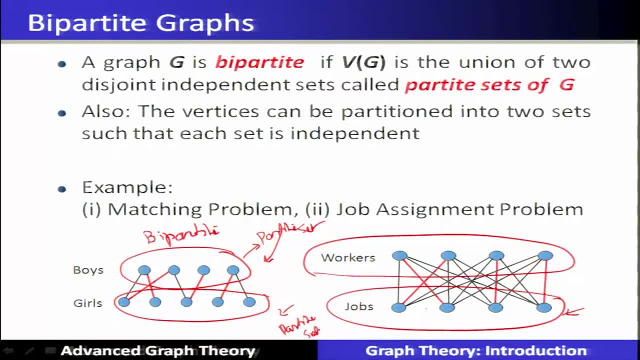 that is called a bipartite graph. So this particular example: you can see that it is written as a matching problem. that means boys and girls. you want to find out a match. match means the set of edges, which will be. basically. this edge will include one boy and a particular girl. 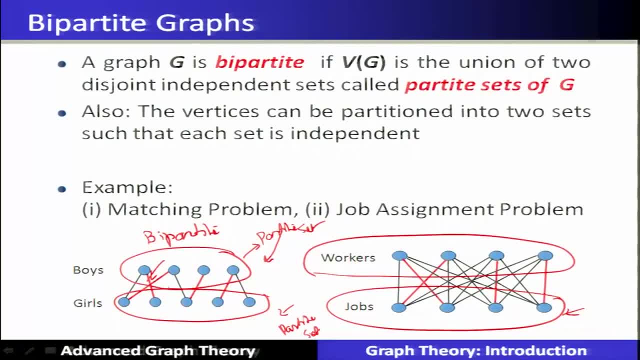 So set of such disjoint edges is called basically the matching. So matching problem is the set ofこ 1, traiterr только 0s and 0s, trivial ogenznil sense. Also, if there is such disjoint edges Consider one chance個eyed stature of that area of the graph C. emotionally it can be predicted for so simply thatże impossible with such inheritance scoring. But if there is any imagination to get that stretch of Yanucki and M Bright. But if such randomness is known only so that should be very difficult as well. 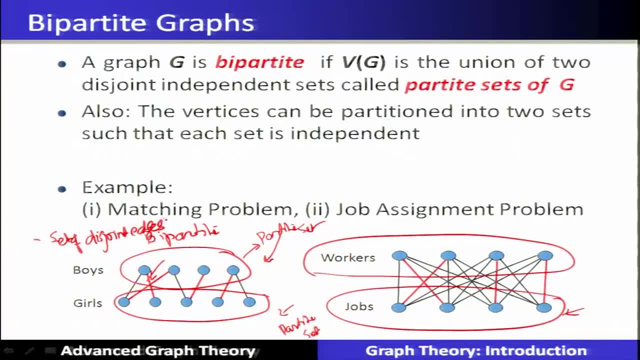 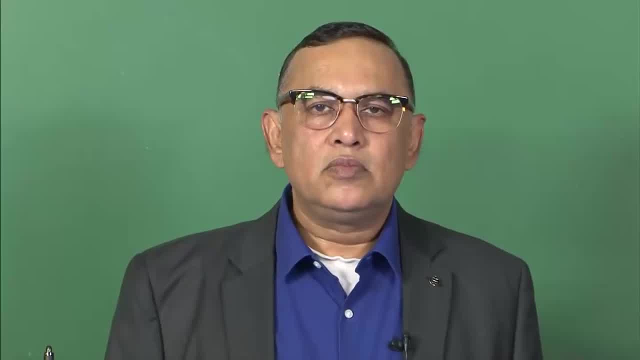 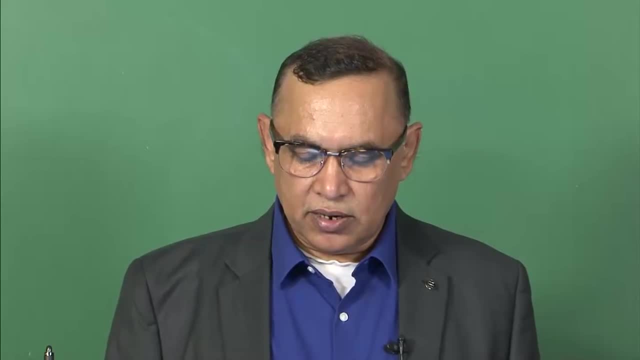 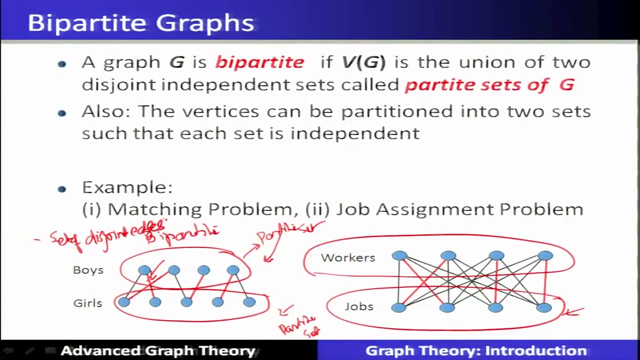 Alright, So you have to find out these set of disjoint edges so that it will solve some problem in an efficient manner and optimal manner. Similarly, job assignment problem also is to find out those set of match or edges which will basically assign the workers to the job so that it will give the maximum profit to 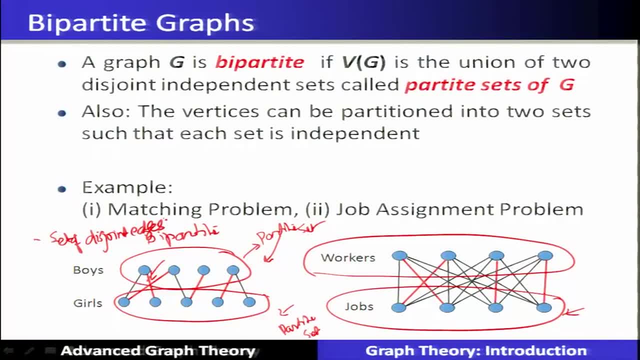 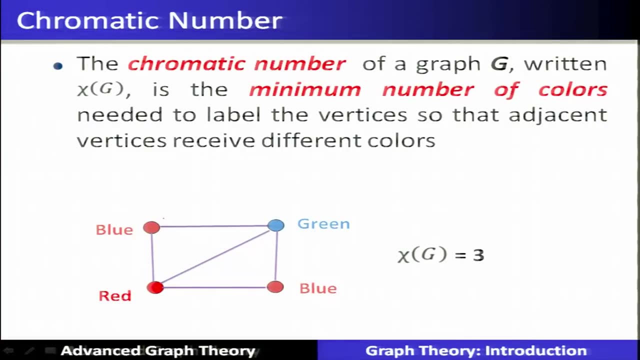 the company. So that is a job assignment problem. Similarly, the matching problem is to match the boys and girls to for a particular purpose or for a particular applications. Now with this partite set- we have seen the two partite sets- is called a bipartite graph. 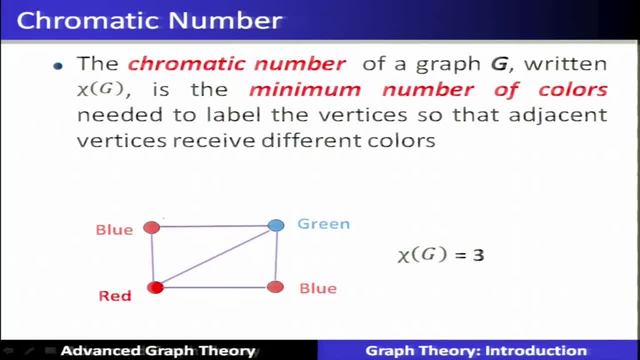 Similarly, if there are more than two partite sets, then we have to define a parameter, or that is That is called the chromatic number. So chromatic number of a graph G is written by chi of G, So this is a Latin symbol. 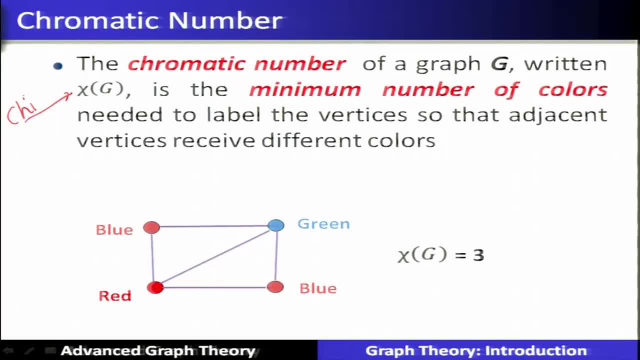 So it is. a chi of G is nothing but a chromatic number of a graph, is the minimum number of colours needed to label the vertices so that the adjacent vertices should receive different colours. So let us take this example over here in this particular graph. 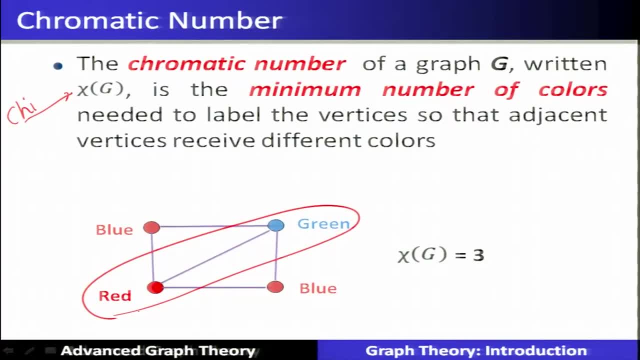 These two edges, which are these two vertices which are basically adjacent, so they are receiving the different colours. These set of vertices, they do not share an edge, so they are non-adjacent, so they receive the same colour. So how many minimum number of colours required to colour the graph so that no two adjacent? 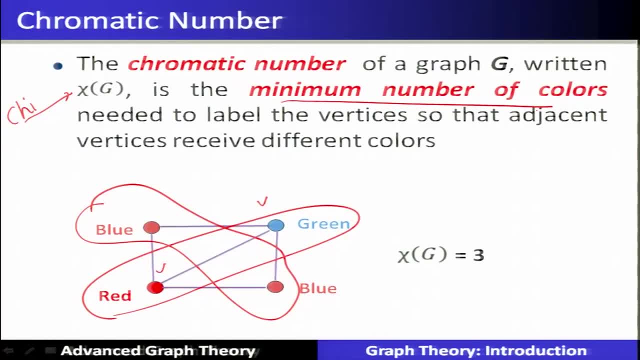 vertices receive the same colour is basically you can count 1,, 2 and 3,. three different colours are required, So the chromatic number of this particular graph is 3.. So you can partition this graph into three partite sets. 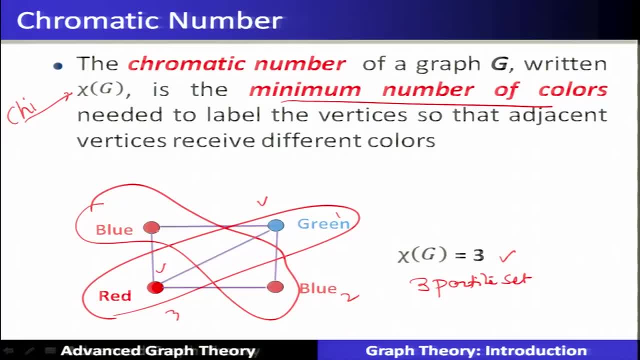 What are these three partite sets? So all the blue coloured will form one partite sets, 1 and 2.. 1 and 2, let us say, then there will be a green, is another partite set with only one vertex. let us call it as 3, and then there will be another set partite set, let us call: 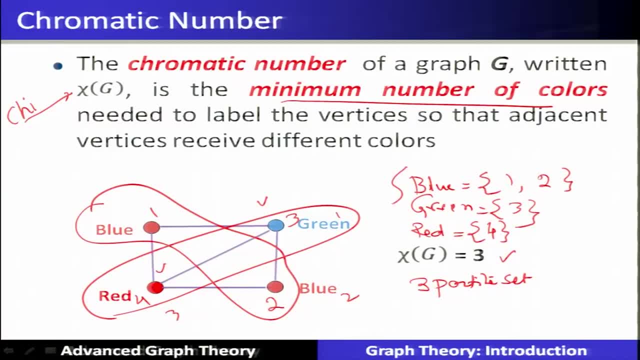 it as a 4.. So it will have the three partite sets. So this particular chromatic number is nothing, but it will partition the set of vertices of a graph into three partite sets. So this particular graph you can see is a generalization of a bipartite graph which 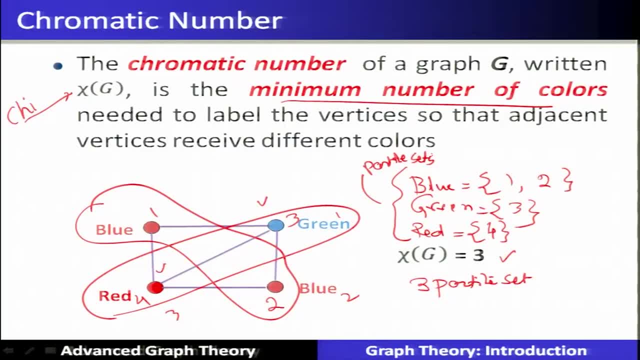 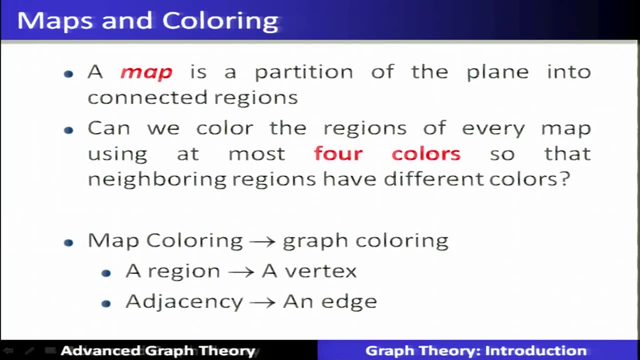 has only two partite sets. here you have obtained more than two partite, that is, a three partite sets, and that particular value is called the chromatic number of a graph. that is represented by chi of g. Now, the maps and colouring of a map is not a trivial problem and it is a well studied. 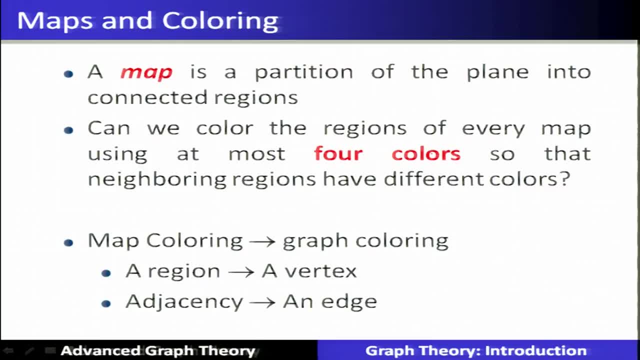 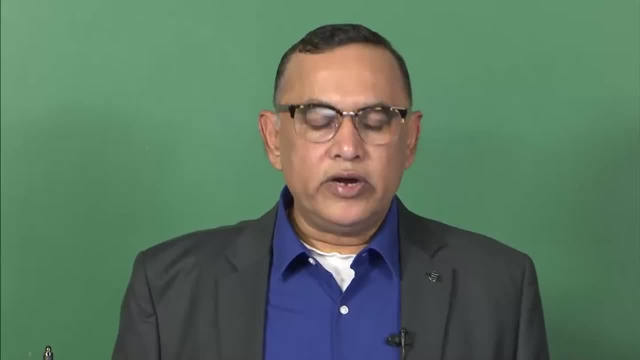 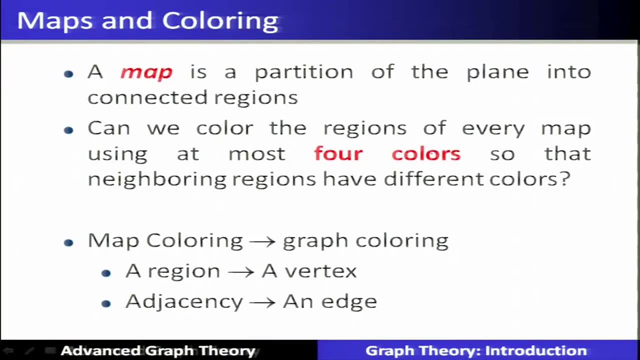 problem in a graph theory. So map is a partition of a plane into the connected region. You might have seen the atlas as an example. So how are you going to colour this particular map using at most four colour is a well studied problem. 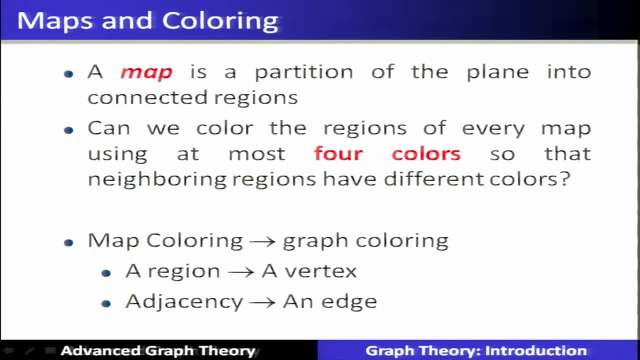 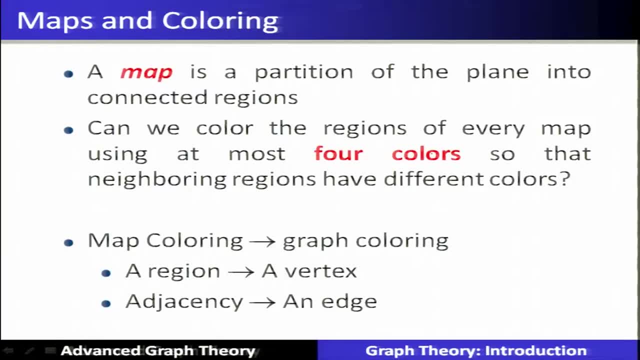 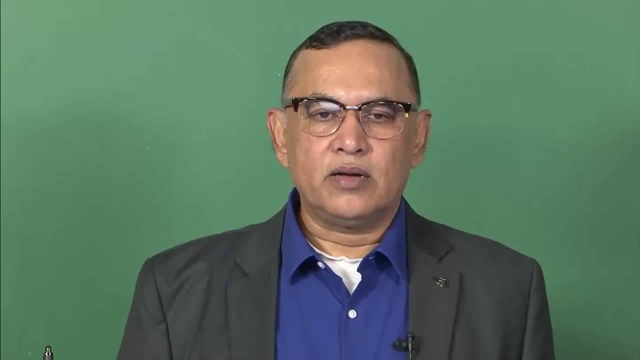 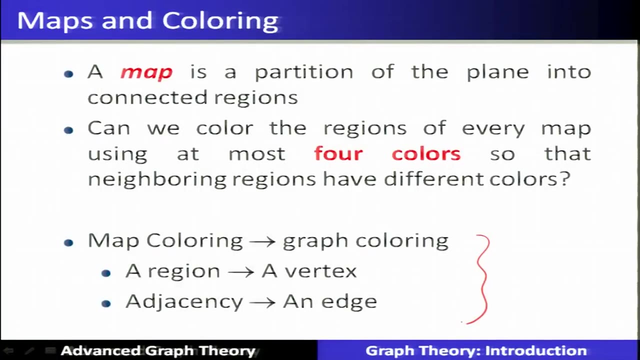 map using at most four colours, so that no neighbouring regions receive the same colours. So any two neighbouring region, they are going to receive a different colours. So how, using four colours, you can solve this particular map colouring problem. This particular map colouring problem can be represented as a graph: colouring problem. 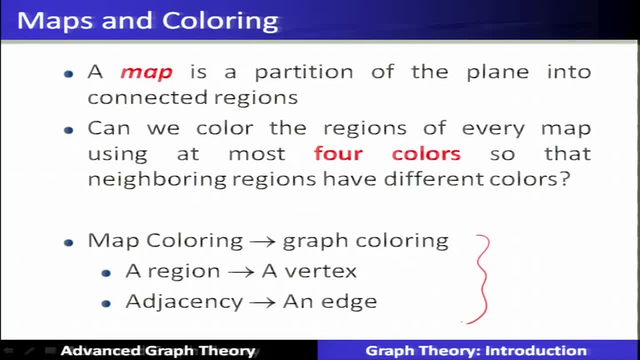 You can see the map colouring problem in the following manner: The regions in a map you can be representing as the vertices of a graph and the adjacency relation between the regions, if you can represent as a edge of a graph, then this map colouring problem can be represented in a form of a graph and map colouring you can represent. 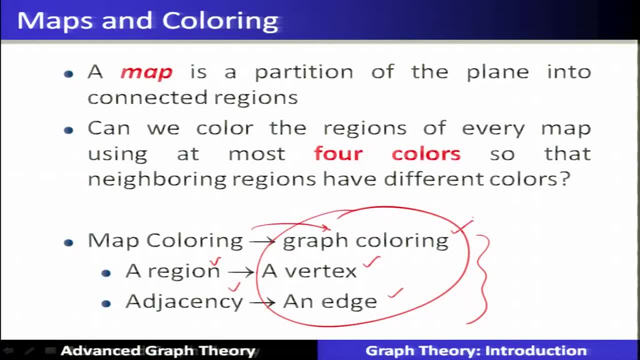 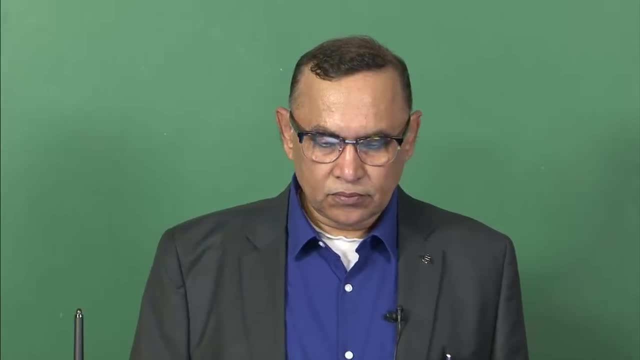 in a form of a graph colouring. That means you can find out the chromatic number of a graph and you can check whether it is at most 4 or not. So that particular problem you can solve using map coloring problem, can be solved using the graph coloring problem. 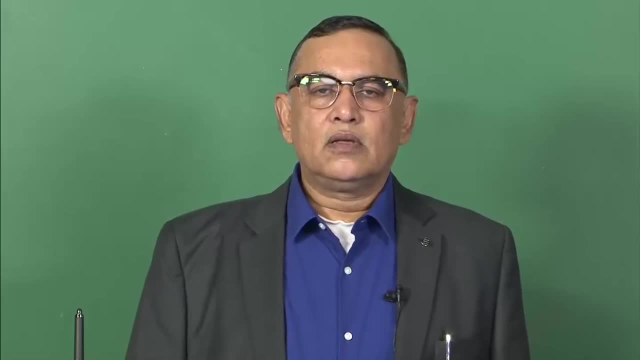 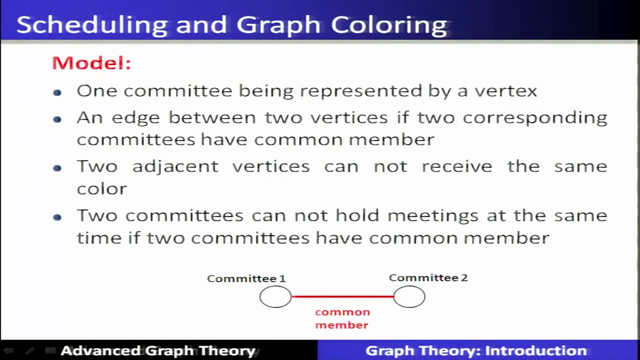 Now we are going to see more applications here and how the graph theory is, a model of a graph- can solve this particular problem efficiently or can analyze the problem to the satisfaction of the solution. For example, let us take the scheduling problem. So we 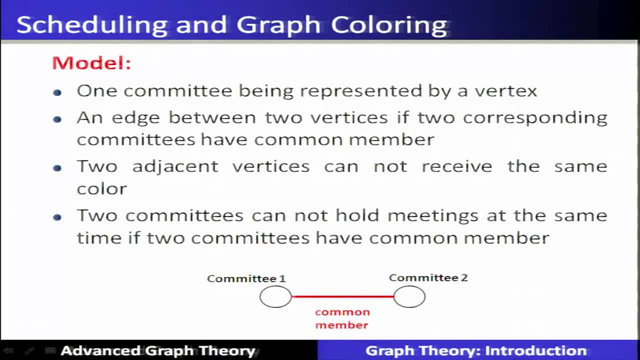 want to find out how to schedule the meetings of different committees with a minimum number of time slots, and this is called a scheduling problem. So this particular problem you can model in a form of a graph, wherein the committees are represented in a form of a vertex, and 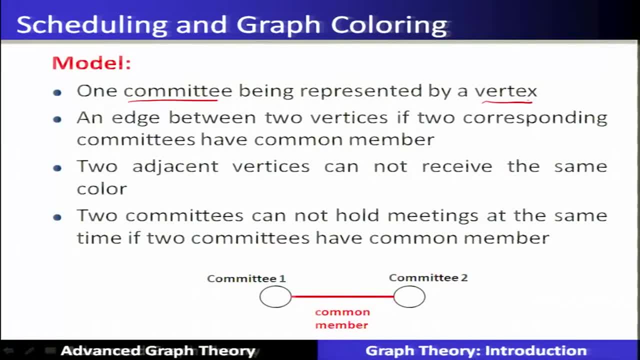 if there is a member present between these two committees, or a particular member which is common into these two different committees, then you place an edge. So edge in this particular graph will represents the committees having a common member. So now here we can see that this particular 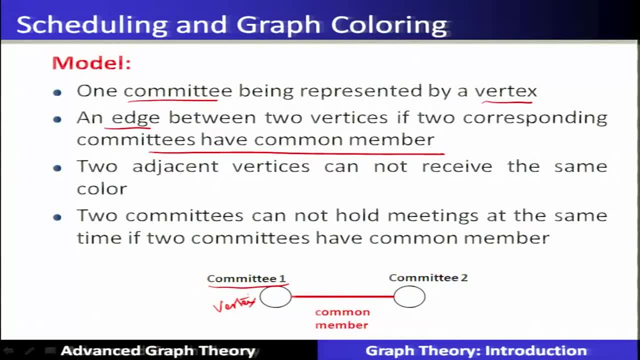 committee is represented in a form of a vertex, So different committees are represented in a form of a vertices of a graph, and between committee 1 and committee 2 there is a member which is common. So basically they are represented in a form of an edge. 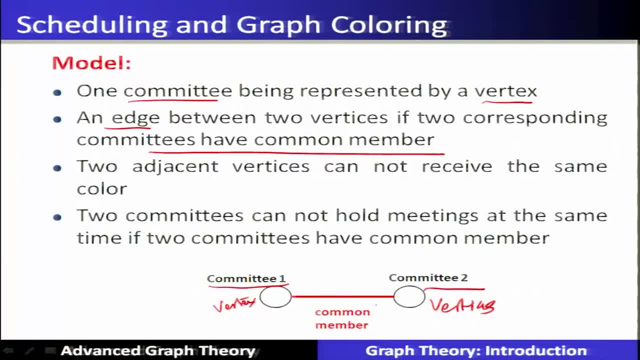 So this: having formed a graph out of the entire problem setting, we can find out the chromatic number of that particular graph. Having known the chromatic number of a graph, we can find out the how many minimum number of time slots required to schedule all the. 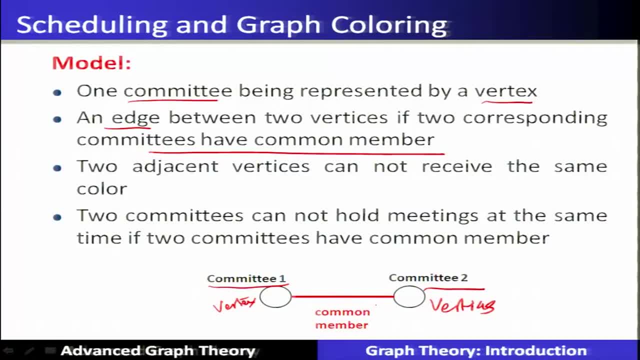 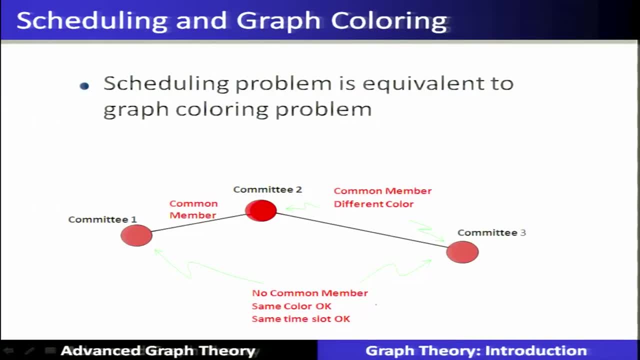 meetings, and hence you can solve the problem In this particular way. So, therefore, the scheduling problem, basically making it as an equivalent to a graph coloring problem. So if you know how to solve the graph coloring problem, we can solve the scheduling problem very well. 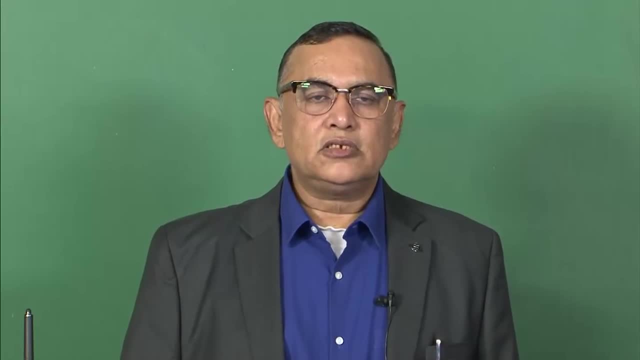 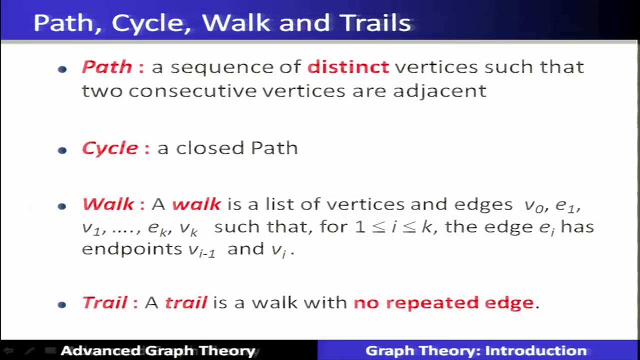 Now let us quickly take up some of the definitions. Those definitions we are going to quickly see their path: cycle walk, trails, path. A sequence of distinct vertices. So we can write it as V char. So is that two consecutive vertices are adjacent, For example V1, V2,. 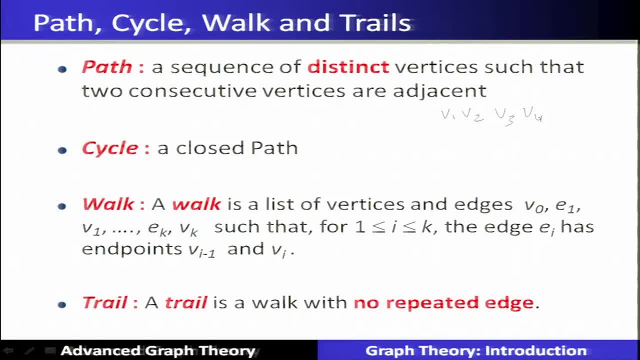 V3 and V4. there are four sequence of vertices. all these vertices are a distinct in the sense they are not repeated again and any of these two vertices are adjacent. that means V1 and V2. they are having an edge. Similarly, V2 and V3 is having an edge. V3 and V4 is having. an edge. various worth of vertices are a set, So a set of vertices are exists. The set of vertices is decreased. thereby everything that you can have is kidding. This definition is tactic to understand. It does not cover the safety and security of a graph drawing. 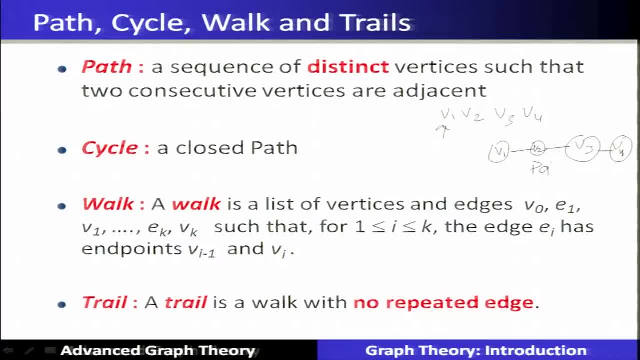 We only see a display of graph this'thave E. That is the actual size though. So, For example, this efficient rate isfter 0 to a Chem. This is what is what is having an edge. So this is called a path. Cycle is a closed path. that means after v4. 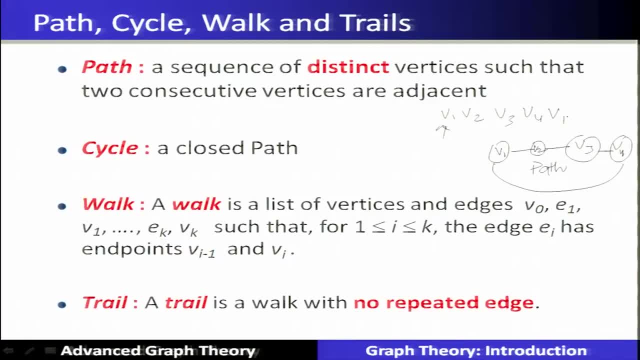 if there is an edge to v1, then it is called a cycle Walk. a walk is a list of vertices and edges such that for a particular edge, ei, it has the end points in vi minus 1 and vi. So, for example, if this edge is ei, e1, e2, e3 and e4. So you can write down the vertex v1, e1,. 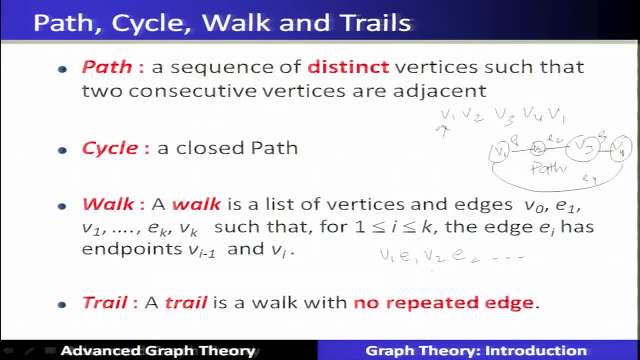 v2, e2 and so on. So for a particular edge, ei, it has basically. So here we have to write down v0, v1, v2, v3 to have this particular notation: v0, v1, v2, v3. 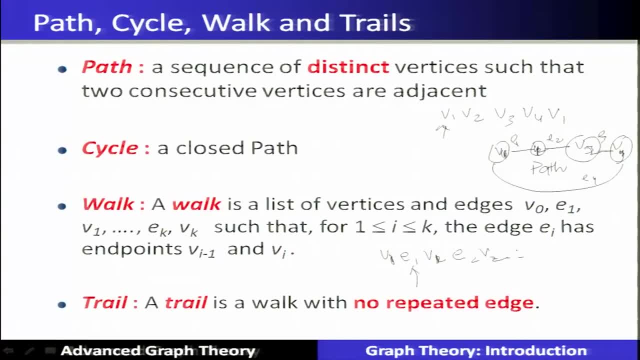 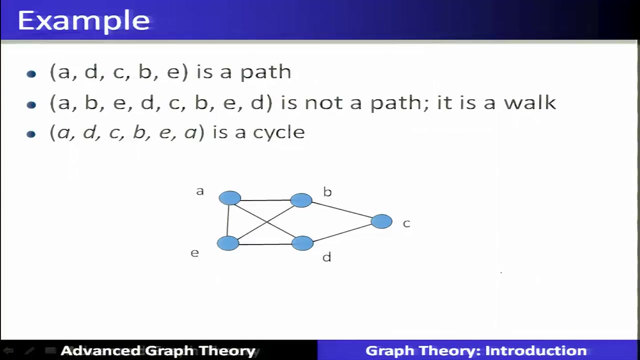 So a particular edge, ei, has the end points as vi minus 1 and vi. So having this kind of list of vertices and edges is called a walk. A trail is a walk with no repeated edges. So if the edges are distinct in a walk then it is called a trail. So in this example, a, d then c, then b, then e. 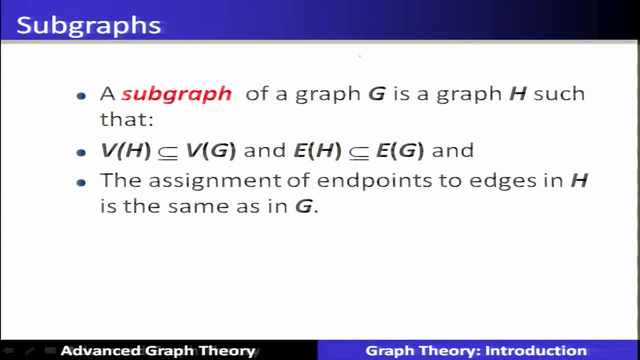 this is a path. Subgraphs. Subgraph of a graph g is a graph h, such that the set of vertices of that subgraph h is a subset of vertices of that particular graph g and the set of edges of the subset of a subgraph h is a subset of edges of a particular graph g And the assignments of the. 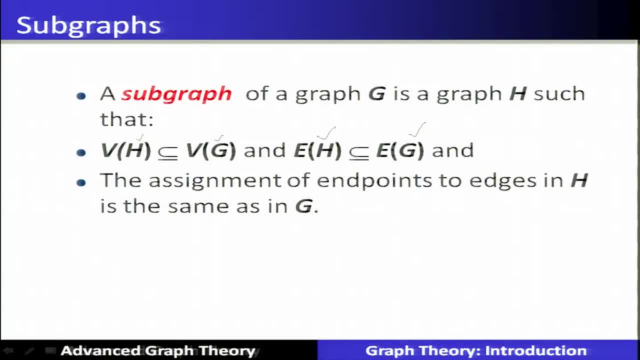 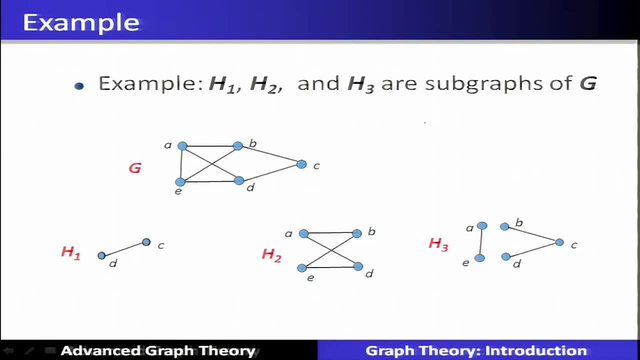 edges in h and is the same as in g, then it is called a subgraph of a, then it is called a subgraph of a graph g and that is represented as an h. So in this particular example we can see here that if this is the graph which is given, then h1 is a subgraph of g. So 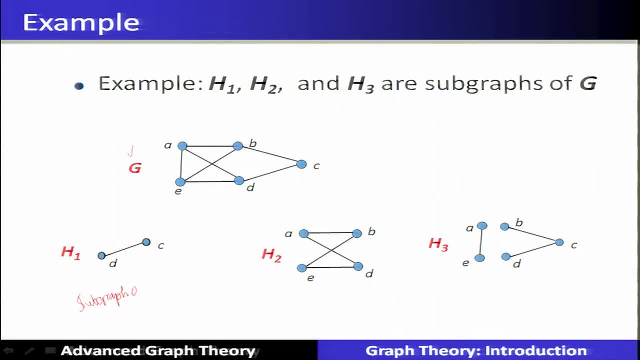 h1 is the subgraph of g, So h1, you can see c and d, So this becomes a subgraph of g. So all the incident edges to these vertices. shove in H1, the incident edges to this vertex H1 fairly. 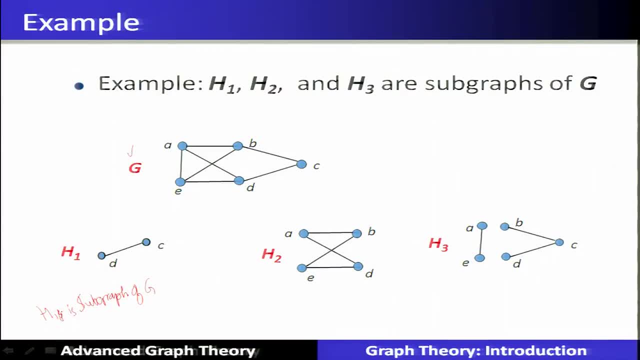 is from the target and g is personal for every vertex because h1, if you küp it from top to the second, Now you follow up h1 appears in letter a and this line 1 is the went. So note the Collins dimension. h1 is this общ phải where h1 is ever expanding. 1 above is the 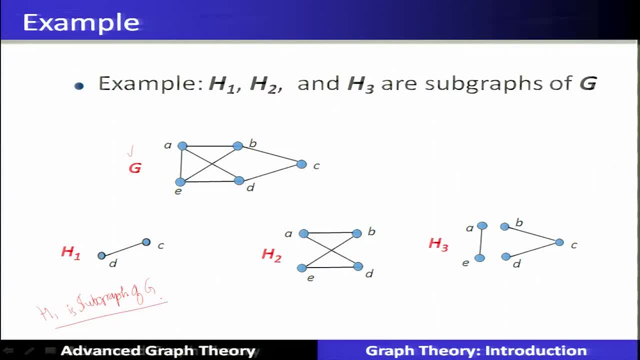 geral situación. 0 is equal to 0 and 1 below it will remain 1 amperes, So the general function is 0 and the total duration equal to 0.. So h2 is 3 chemical operations, So the general Cristian Zun невay per square millimeter and 1 over h2 equal to 0 is equal to: 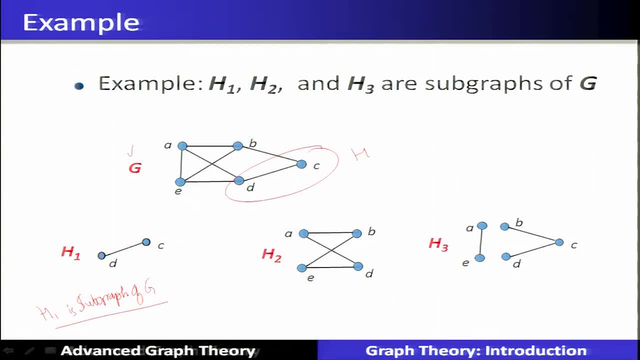 the incident edges to these vertices is basically of a sub graph. H 1 is also present in the main graph, Hence it satisfies the definition of a sub graph. H 2 is also is a sub graph of G. So H 2 is a graph and it is also a graph. So H 2 is a sub graph of G. Now we 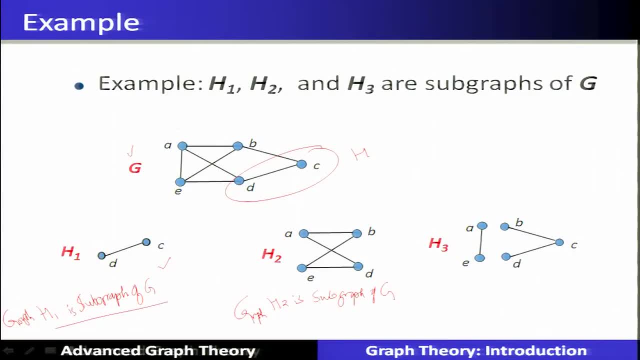 can see A, B and E D, So A, B and E D, So the edges which are present, this is not present. So all the edges which are present in H 2 are also present in G, Hence this particular. 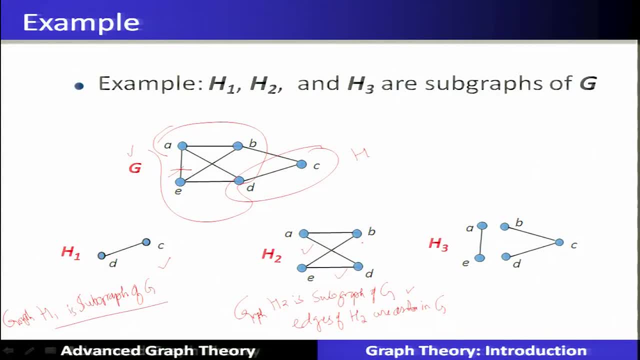 and also the set of vertices which are present in H 2 are also basically the subset of the vertices of G, Hence H 2 is a. hence the graph H 2 is a sub graph of G. We can see that A, E. 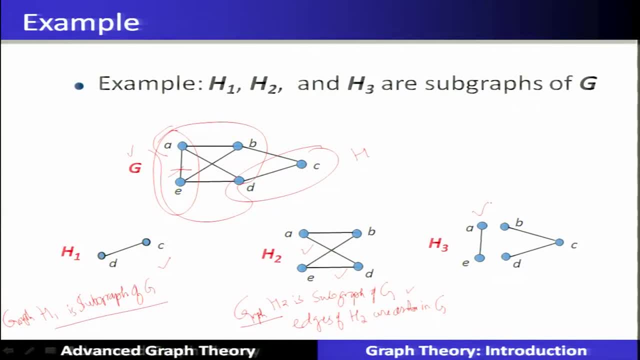 This edge is also present. vertices are also present in G, Similarly B, C, D. this particular component is also present. Hence the entire graph, that is, the graph H 3, having two components, is a sub graph of G. So we have seen the definition of a sub graph and some examples. 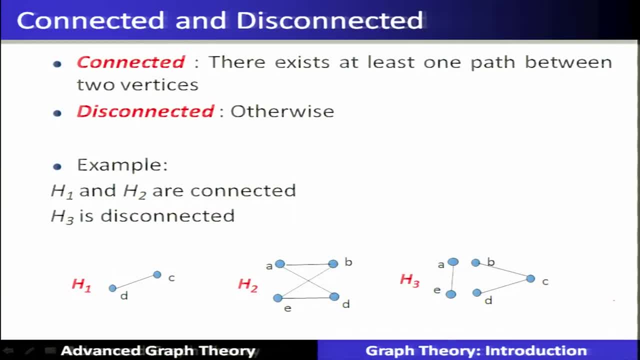 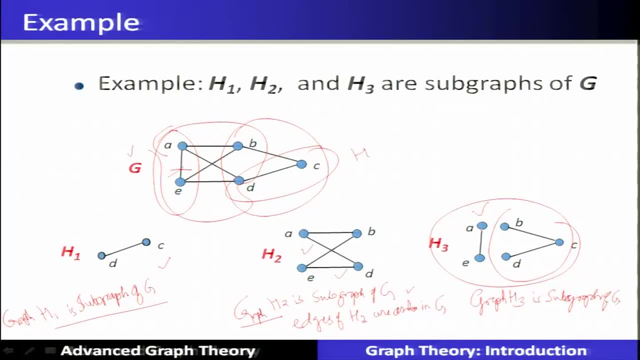 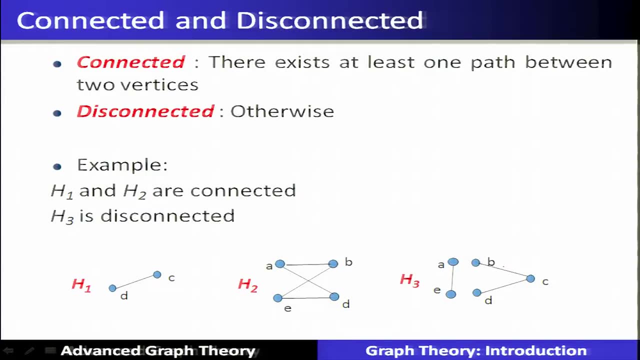 Now we are going to see the definitions. some more terms and definitions Here. we have seen that the graph H 3 has two components. it is not a connected graph. So therefore we have to see what do you mean by a connected graph. 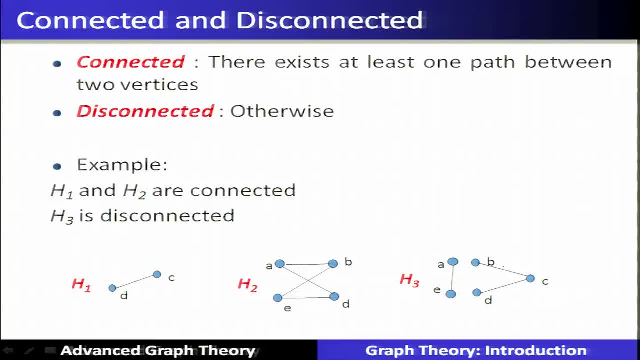 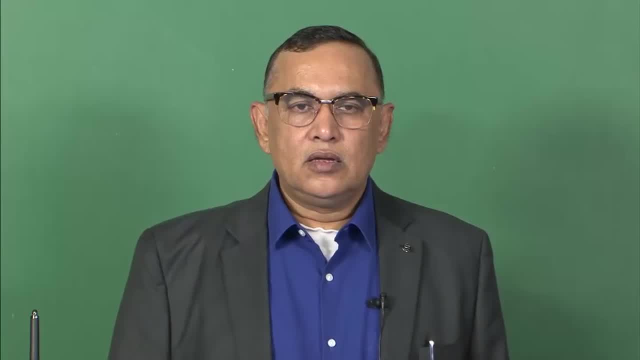 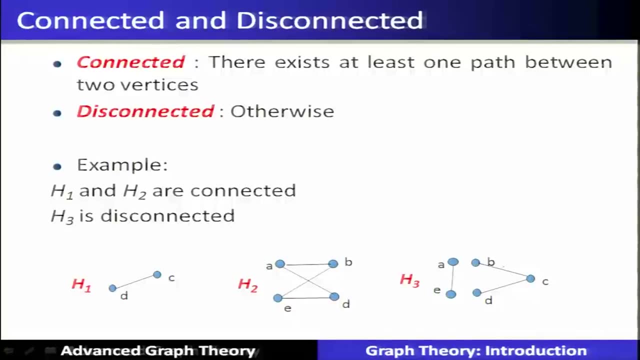 So a graph is connected. if for every pair of vertices there is a path, Then that graph is called a connected graph. Otherwise it is disconnected. So the example of H 3 is a disconnected graph and this is a connected graph, and this is a connected graph. 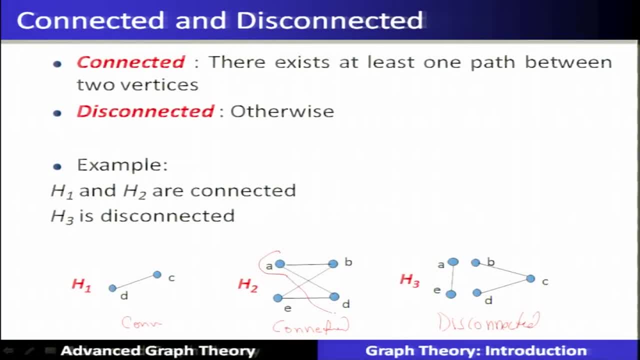 So if it is connected graph between any pair of vertices, there is a path. Similarly, between A and E there is also a path. For example, A is connected to E1.. Thank you to E via D. or A is connected to E via B. So there is a path between A to E. So there. 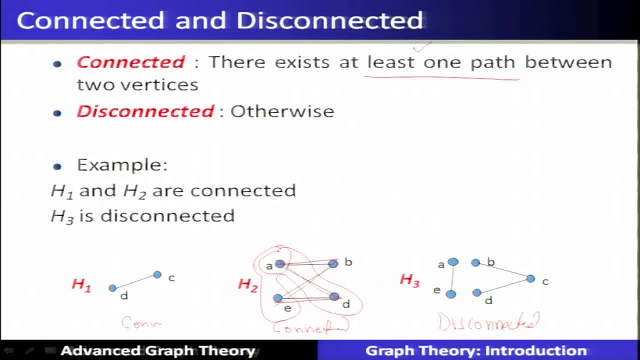 are more than one paths, but it says that at least one path exists between a new pair of voltages, So that exists. hence S2 is basically a connected graph. So H1 and S2, they are connected graph, whereas S3 is basically a disconnected. This is very important definition. 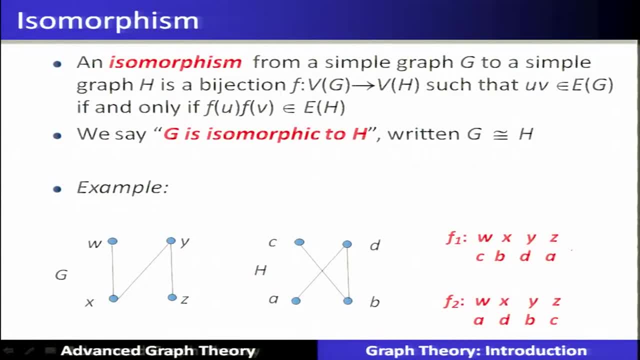 to be noticed. Now, another important concept here is called isomorphism. That means the graphs. you can form the way you like to form. Take this example, the graph G. you can represent this particular graph G in another way. So that means W. 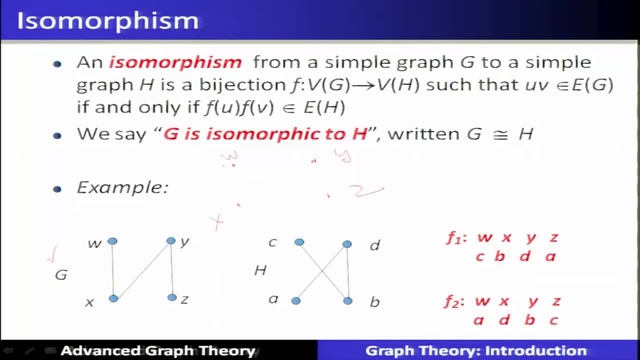 X, Y and Z you can represent using an arc like this, And this arc will also go like this, and this is an arc. So both these graphs are isomorphic in the sense that this particular connection between W and X either you can represent using 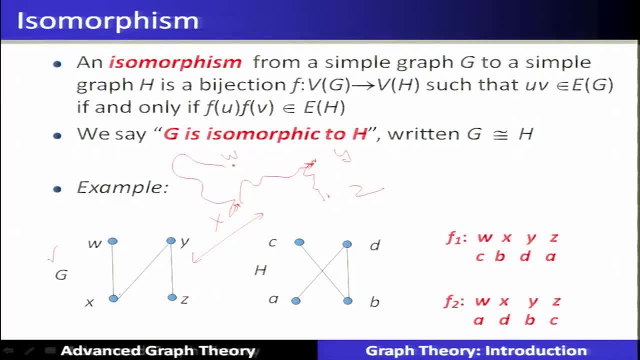 a line or you can represent as an arc the way you like to have. all these connections are preserved in the other graph, So all the relations and all the voltages are preserved. then it is called a isomorphic. So this, called as G, is isomorphic to another. 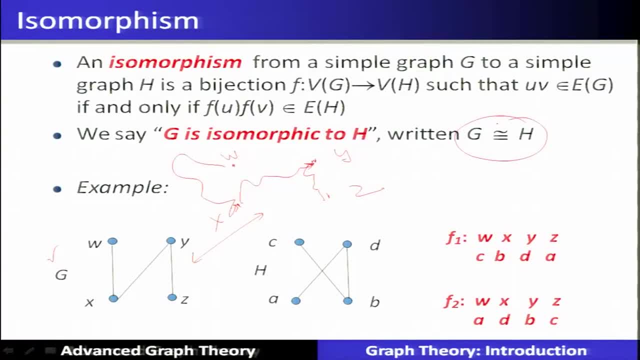 graph and is represented by this particular notation. So whenever there is isomorphism between two graphs, that means there exist a bijection function, F, which will basically do a mapping from the set of voltages of G to a set of voltages of the another isomorphic graph, that is, H. 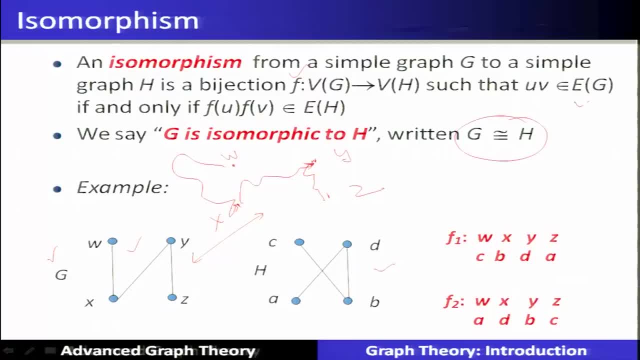 such that any edge which is present in G will implies, or by implies, that that edge in that corresponding mapping to the to another graph H should also be present as an edge. So that means all the adjacency relations are preserved by that bijection function. So if you can, 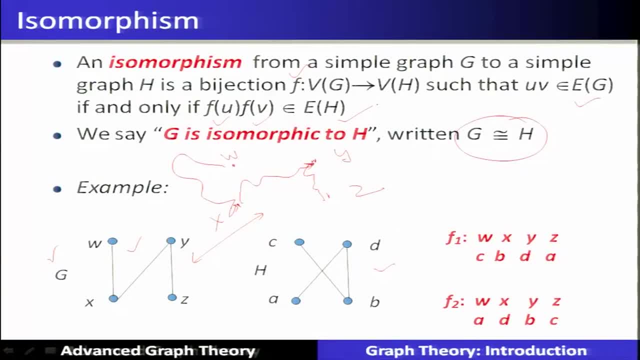 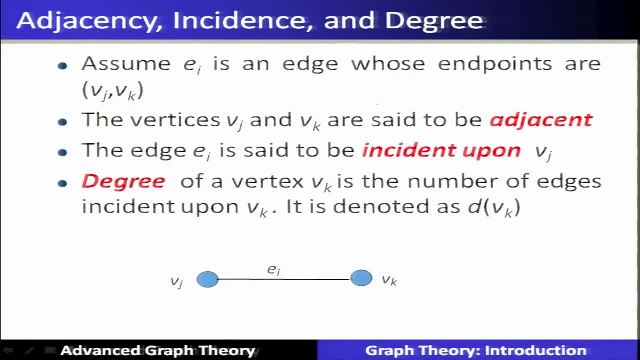 come out with a bijection function between two such graphs, then those graphs are isomorphic and they are written in this particular manner. Few more definitions, as I told you that the adjacency relations are preserved by a function in isomorphic, isomorphic graphs or using isomorphism. 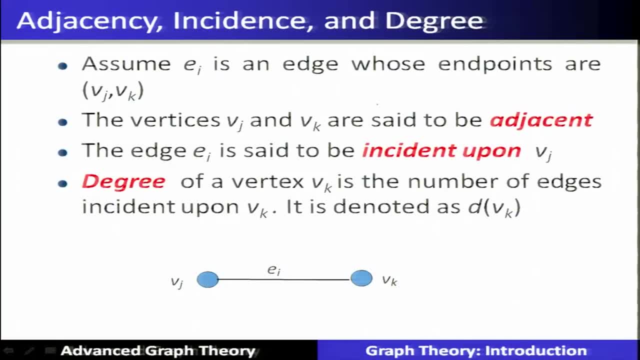 So we are going to see adjacency, incident and incidence and degree, these three definitions, Now the vertices J and K. they are called adjacent if they have an edge which connects both these particular vertices, котораяotiveachancein both these particular vertices、uu note. 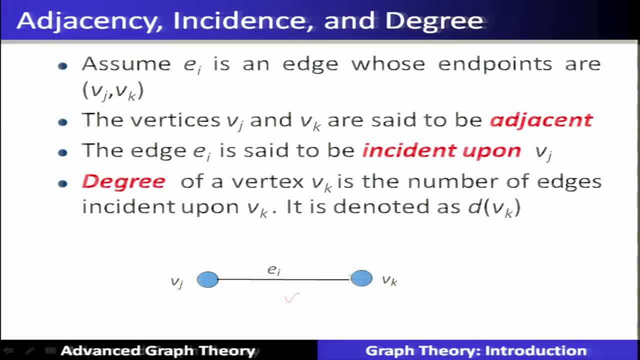 nοEa needlework, that edge is said to be an incidence upon this particular vertex and this edge. you can say that this edge is incidence on this particular vertex. So degree means degree of a vertex, Vk, gm, the number of edges which are incident upon v, k and is represented by that degree of v. 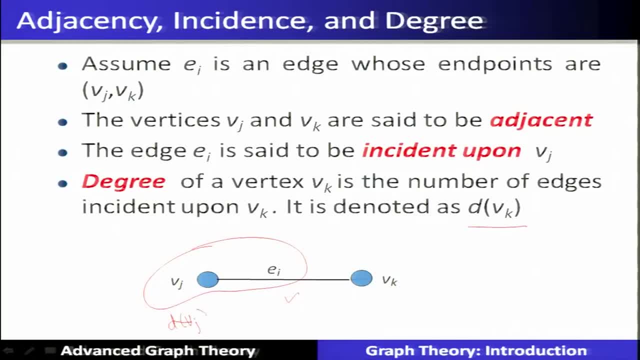 k. So let us take the degree of v? j is nothing, but how many edges which are incident? here we can see only one edge, E i is incident, So the degree of v? j becomes 1.. So whenever we are counting the degree, we are basically finding out the incidence: how many edges are? 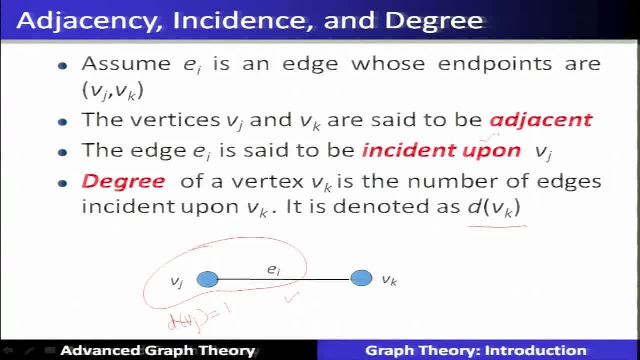 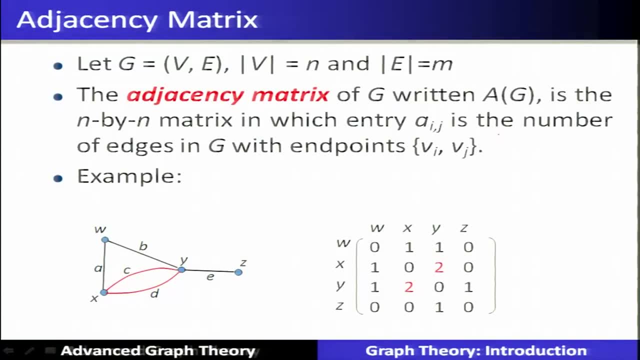 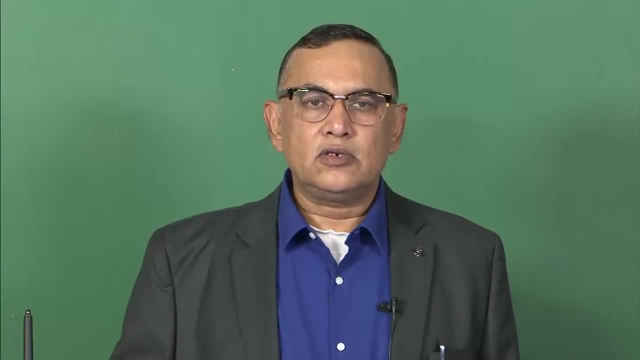 incident on that particular vertex and that becomes a degree of a vertex. I told you that the graph can be represented in a suitable form so that it can be stored in a computer memory. So we are going to see what are those suitable forms. One way: 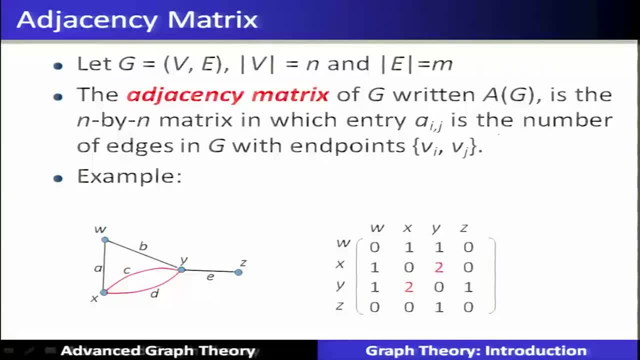 you can represent a graph that is called adjacency matrix. So, given a graph G, V, E having an n vertices and m edges, We can form an n by N by n, by m matrix, and that matrix is called adjacency matrix, wherein each element, a, i is the number. 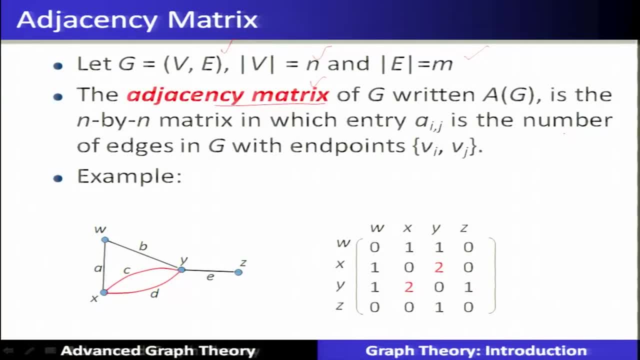 of edges in G with the end points between v, i and v j, For example, y and x, y and x. So y and x, if you take this particular example, x and y. So between y to x, there are 2 different edges which are basically having the connectivity. 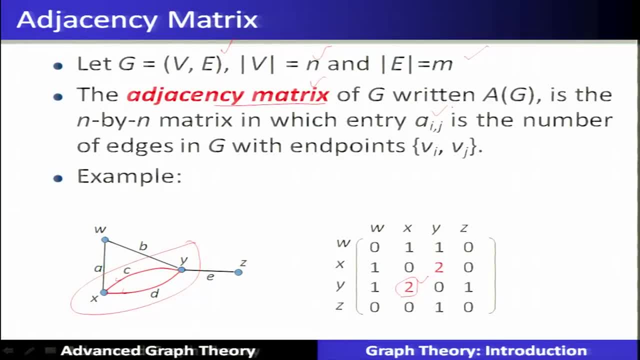 So a i, j entry will be 2.. Similarly, x to y is also 2 i because from x you are having 2 different edges between these end points: v i and v j. So on the row the set of vertices. similarly, on the row also set of verticals. 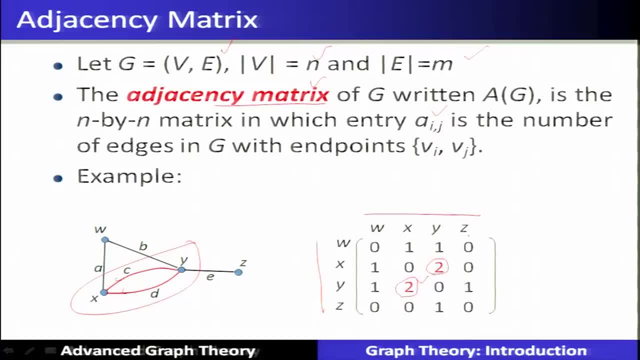 lect powiedział of vertices. these vertices, how many edges basically are connecting them, how these edges are, how these vertices are connected, and this particular connectivity of this representation of a graph is called adjacency matrix. So this is the adjacency matrix representation of this particular graph G. 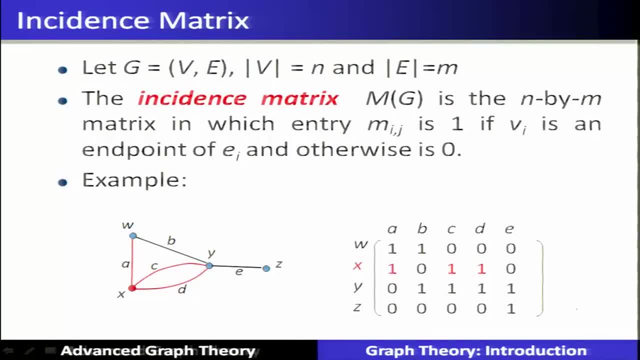 Now another way we can represent and store the graph: in a computer form or in a memory. computer memory is called incidence matrix, Incidence, matrix, incidence. I told you that a particular vertex Vi, how many edges are incident, that relation is being modeled. 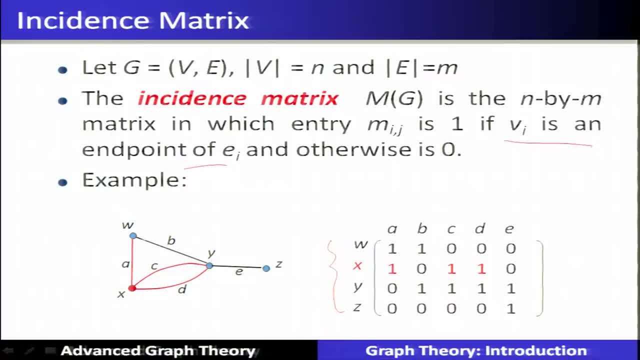 So on one side it will be a set of vertices. on the other side it will be a set of vertices. So on one side it will be a set of vertices. on the other side it will be a set of vertices. So, for example, X is a vertex. so you can see that A is incident on edge or A incident. 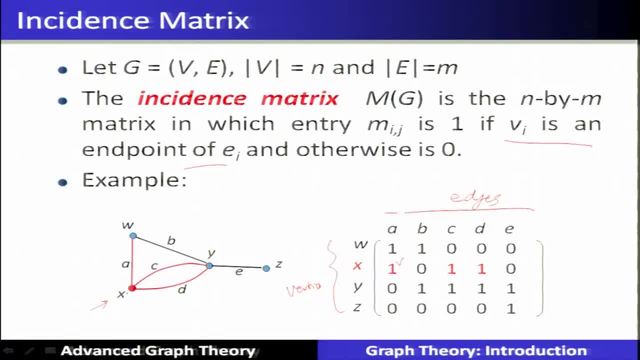 on X, so it is 1, then C is incident on X, so it is also 1, and D is also incident on X, so it is 1.. So such a representation is called the incidence matrix of this particular graph G. 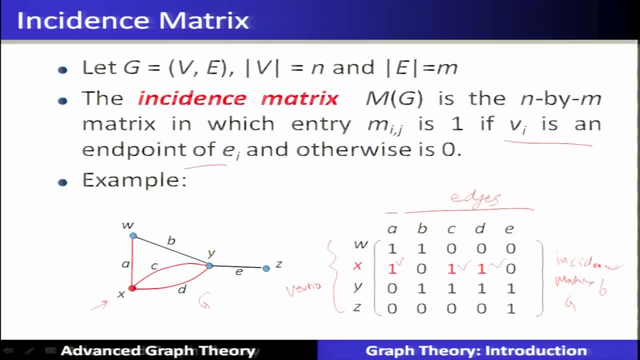 There is one more way to represent the graph. that is called adjacency list, representation of a graph. For example, this is the graph. so for every vertex- X, Y, Z, W, you can find out the list of nodes or vertices which are adjacent. 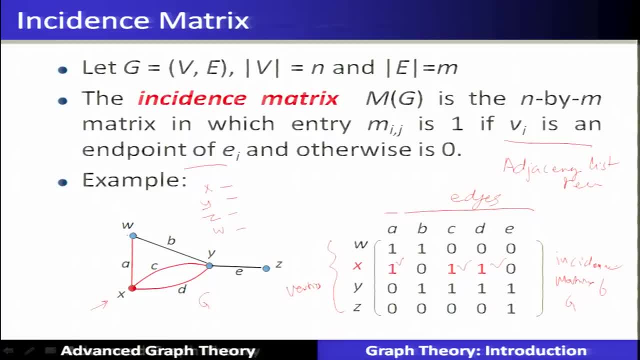 For example, X will have its adjacency list as Y, So W then Y, then only W and Y. it is basically adjacent to. similarly, Y is concerned: it is adjacent to W, then X and then Z. Z is adjacent to Y and W is adjacent to X and Y. 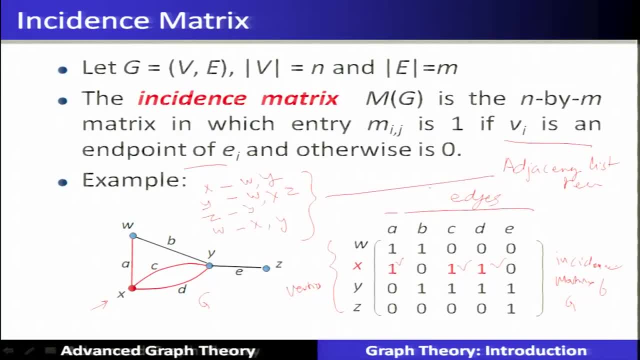 So such a representation is called adjacency list representation of a particular graph. Now you can see the all three representations You can easily express as a data structure in any of the programming language matrix. you can also express and adjacency list you can express in the form of a linked list representation. 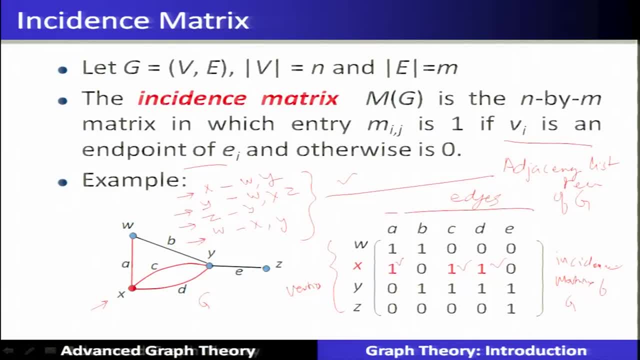 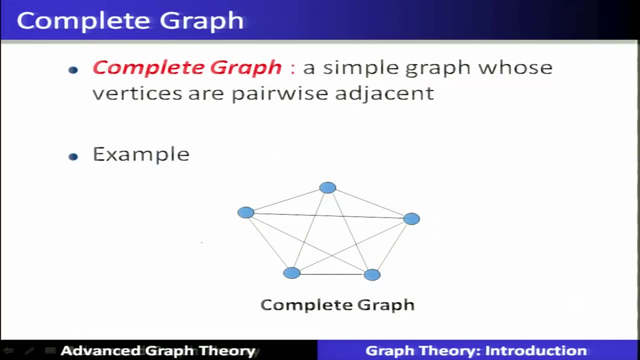 and basically the graph is represented in this way and thereafter you can apply the graph theoretic algorithms, which we are going to discuss In this part of the course. we have seen one graph that is called a bipartite graph. we are going to see another graph, which is called a complete graph. 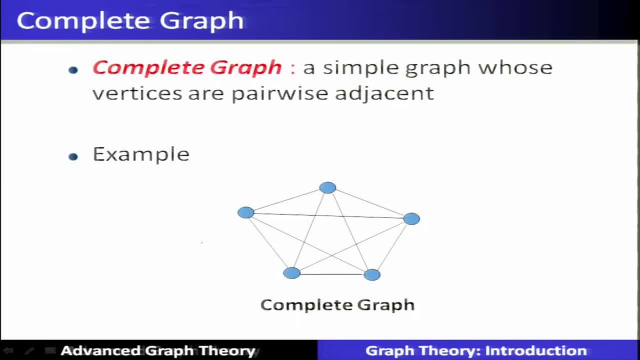 So complete graph is a simple graph whose vertices are pairwise adjacent. So here, in this particular graph having five nodes, all these vertices are basically pairwise adjacent. So pairwise adjacent means this vertex is adjacent to any of these pairs. you see that. 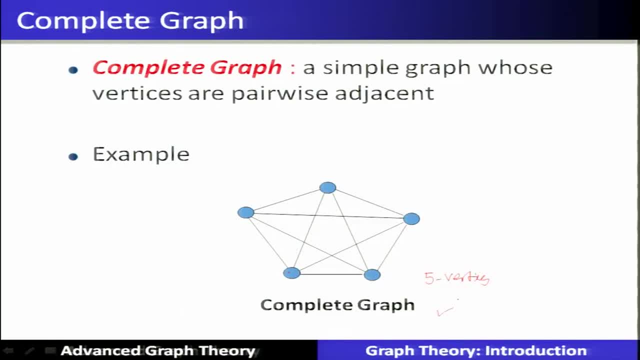 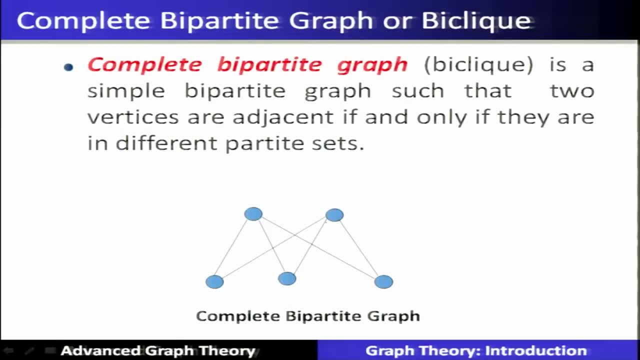 there is a connection, So also all the vertices. Hence it is called a complete graph. Now, complete bipartite graph. it is also called a biclick If it is a bipartite graph and having the adjacency relation to all other vertices. 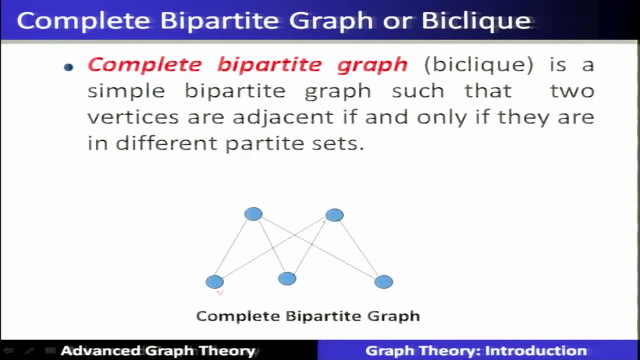 so, for example, this vertex is adjacent to all other vertices on the other partite sets. Similarly, this vertex is having the adjacent to the other partite set, similarly this one, Similarly these vertices are also. hence it is called the complete bipartite set. 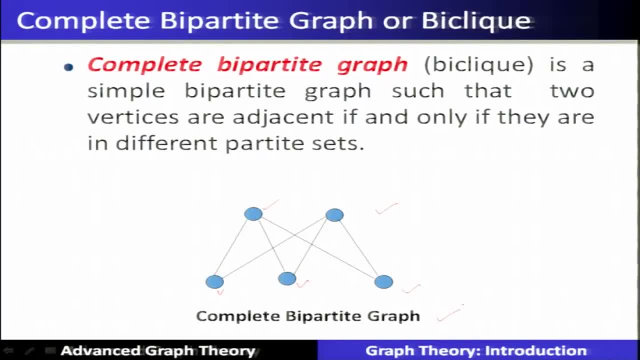 So complete bipartite set is a simple grioskais graph. bipartite set, simple bipartite graph, so that two vertices are adjacent if, and only if, they are in different partite sets. Now another special graph which we are going to just mention is called a Peterson graph.